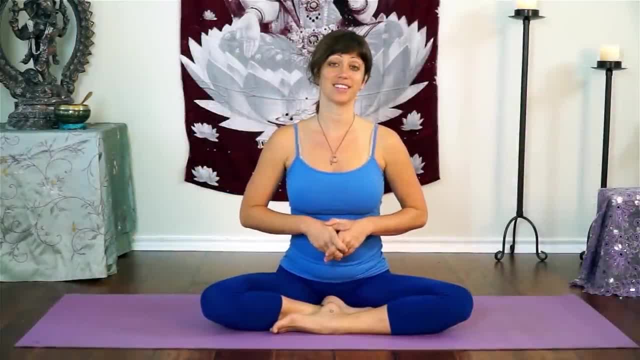 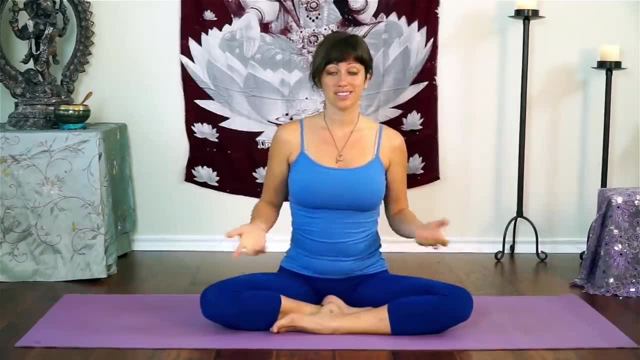 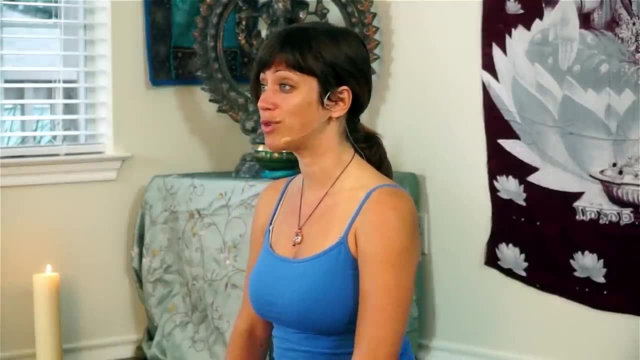 So we're starting from a comfortable seat and it's great to note that we do spend a lot of our time sitting, Sitting at our desk, sitting on the couch, even sitting in your car, sitting in traffic. I know a lot of you commute and have a long drive to work. 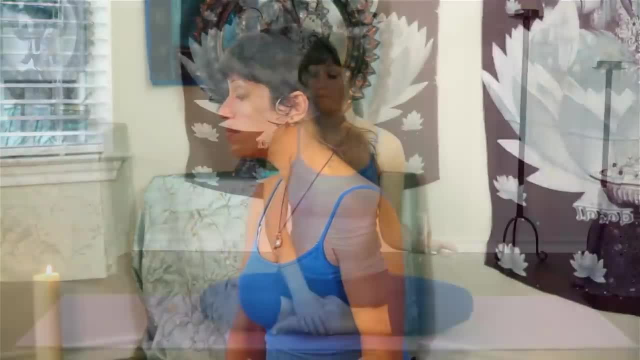 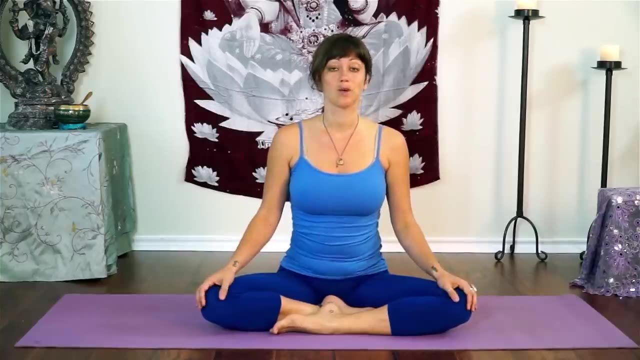 And I'm wondering: do you live close to your job or do you live far away and you spend a lot of time commuting? It's different for everybody, But these stretches that I'm going to show you are really awesome. pretty much anywhere, anytime. 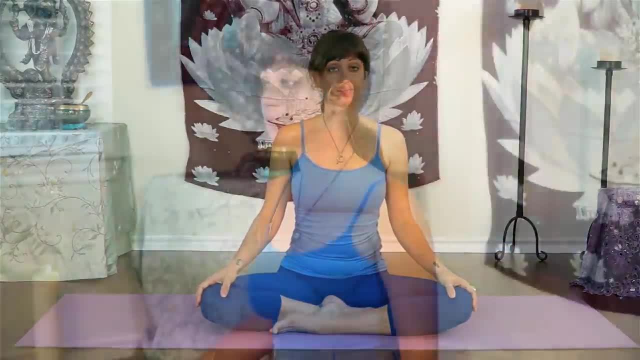 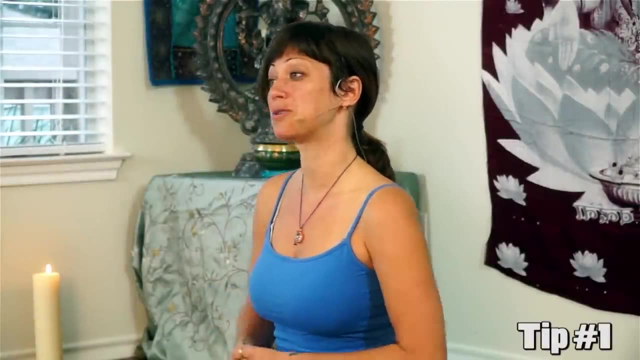 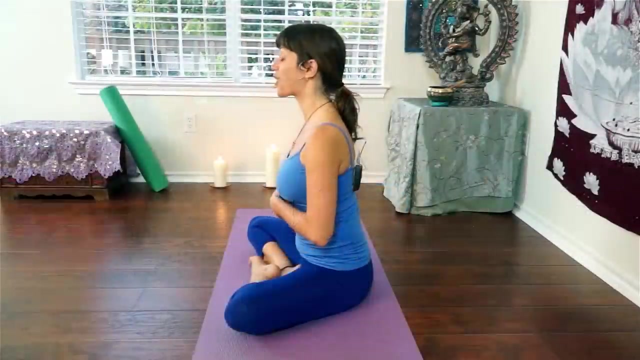 You can do these stretches anywhere, anytime. You can do these stretches to help relieve your back pain. I'd also like to start by telling you my first tip for reducing back pain is to think about your breath and to breathe deeply, consciously. So that's where we're going to begin with our exercise today. 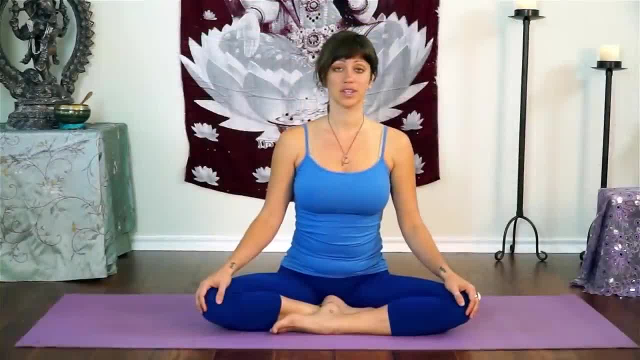 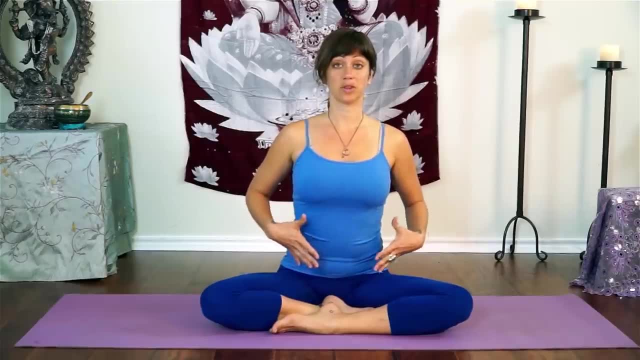 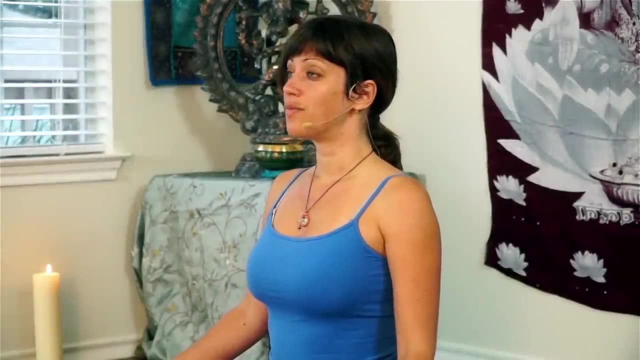 Just by taking some deep breaths. So start by breathing in through your nose, Feel your lungs expand and feel your belly expand as you fill up with air. Then, starting with your abdominals, compress your belly in and breathe out through your nose. 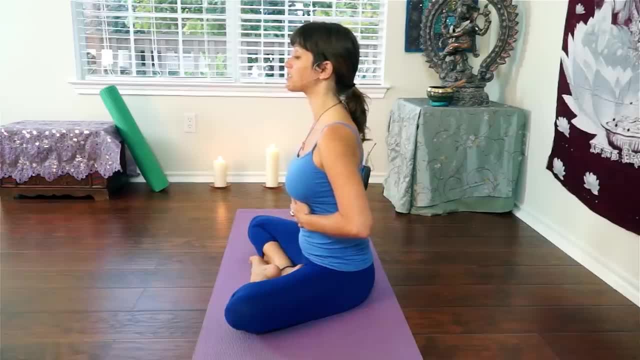 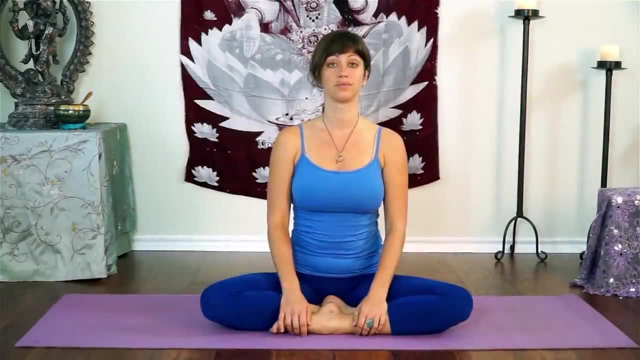 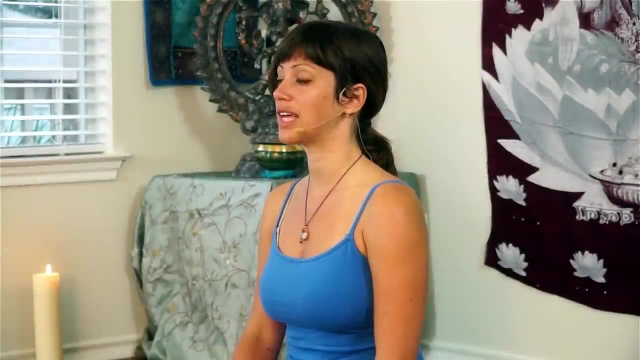 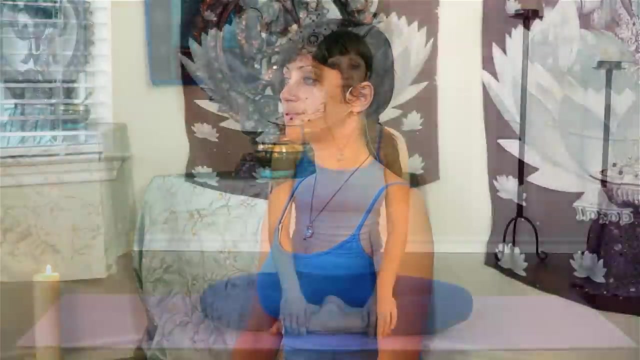 Feel your ribs and lungs compress all the air out and try again breathing in, filling up your lungs And breathe from your belly as you exhale And continue like this, taking a few more deep, conscious breaths. The great thing about breathing deeply is that it forces you to open your chest and 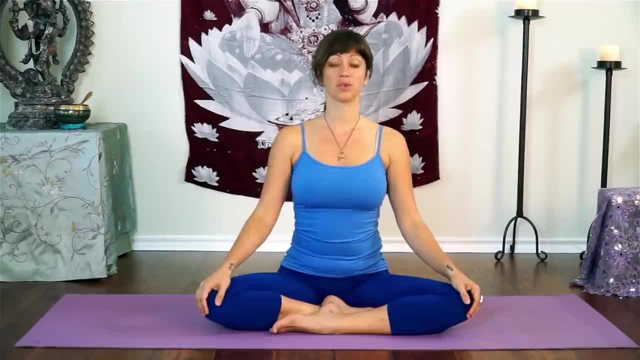 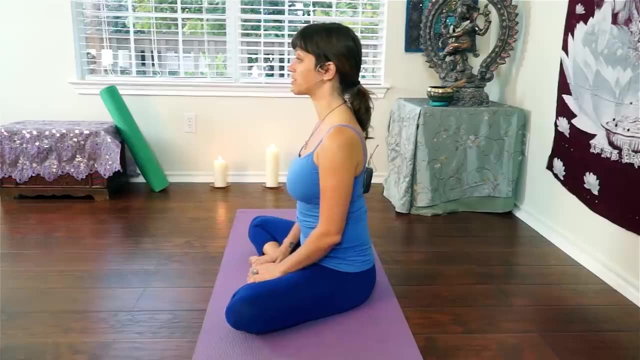 expand your ribs in all directions, So it forces you to take a stronger, more supportive posture, And posture is one of those things that contributes to back pain. So just by simply taking some deep, conscious breaths, you automatically start to improve your posture and reduce your back pain. 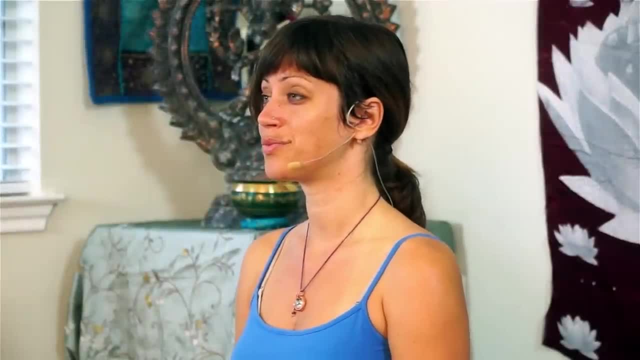 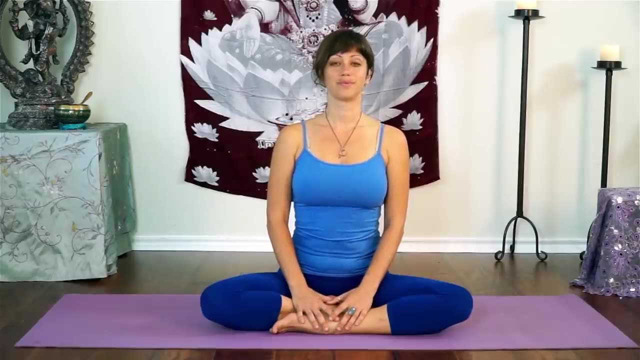 Take one more full breath in and out. See if you can stay connected to this deep sense of rhythmic breathing throughout the rest of this video. We're going to get into some movement now by moving your head from side to side, lowering one ear to your shoulder. 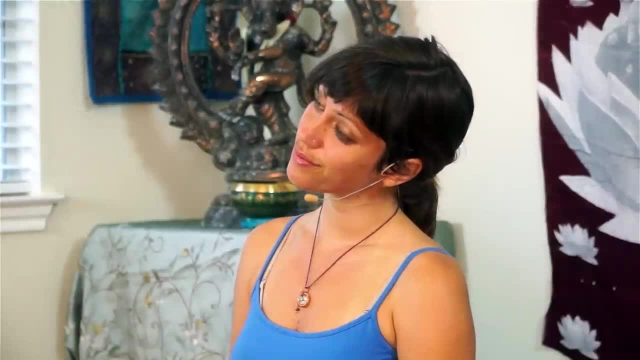 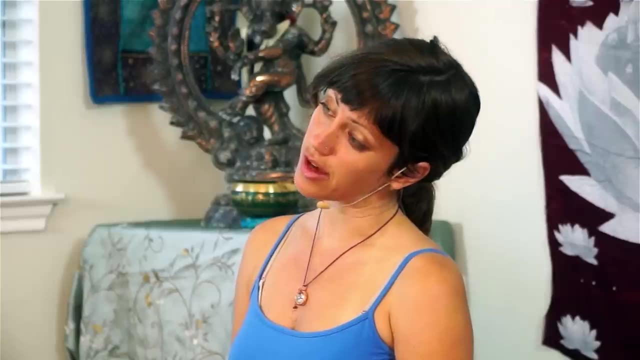 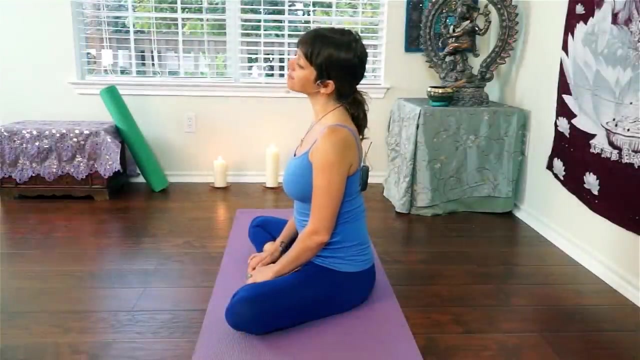 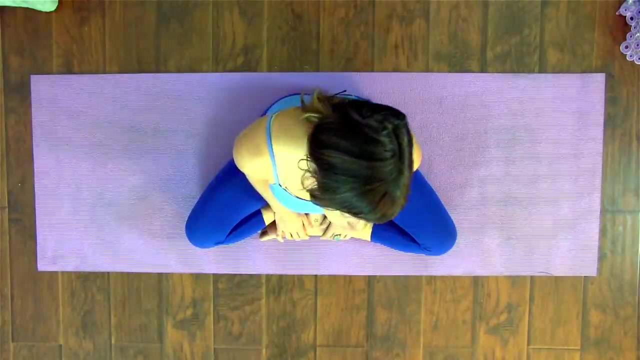 And then to the other side. So we're incorporating some movement, Just allowing the joints in between your vertebrae to start to get lubricated and starting to feel a gentle stretch on either side of your neck. You can move at your own pace. 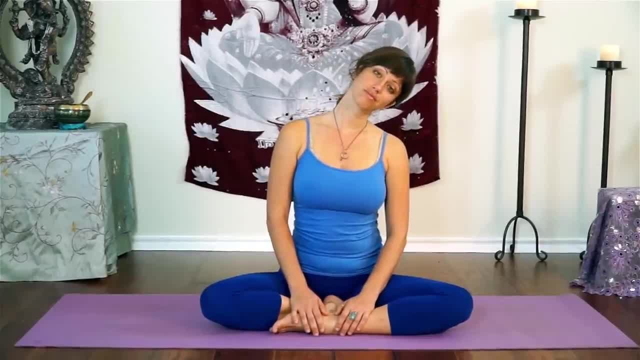 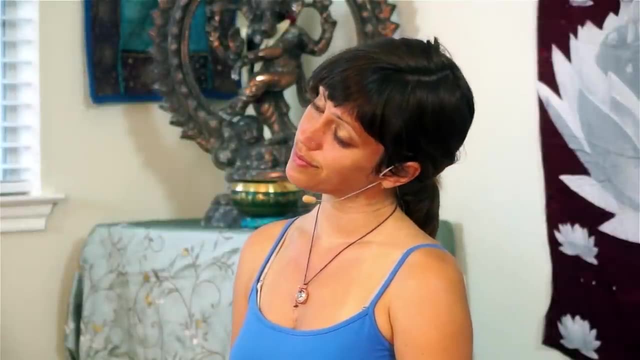 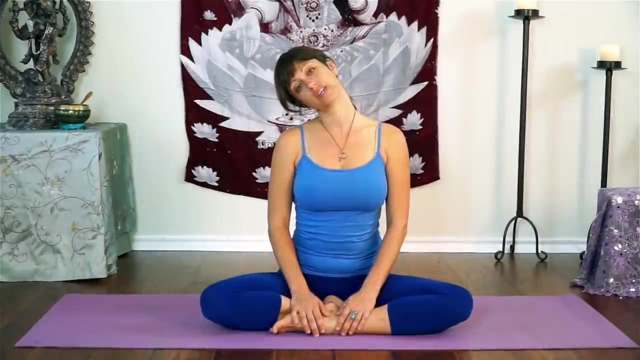 Just noticing where it feels good, Notice where it feels tight, And with each movement you may be able to stretch a little bit farther. Now go ahead and bring your right ear to your right shoulder, and we're going to pause here, Deepening into this stretch. 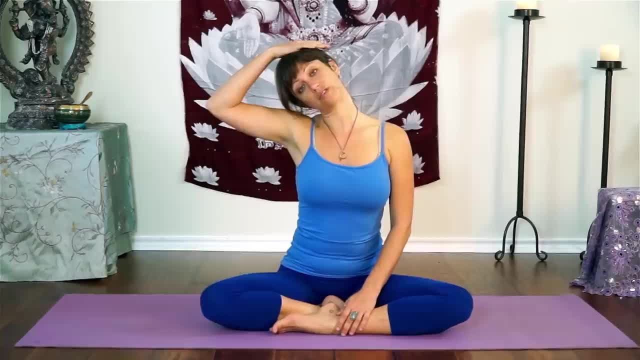 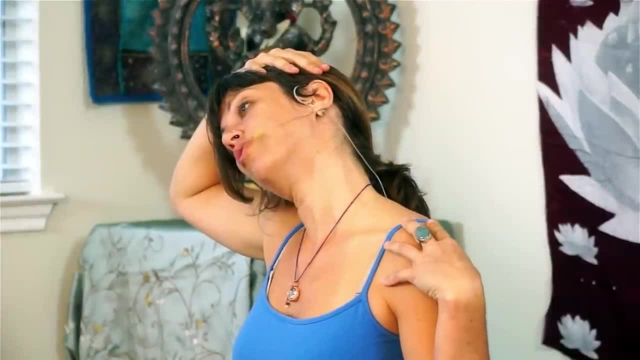 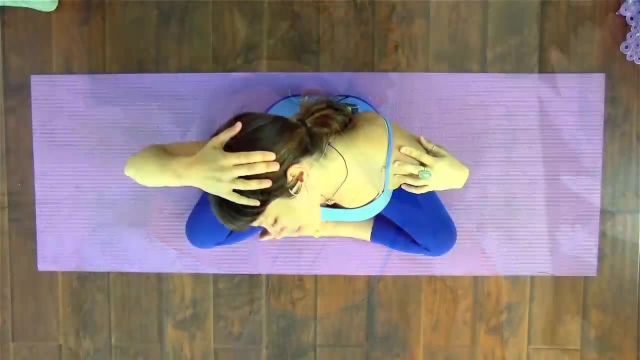 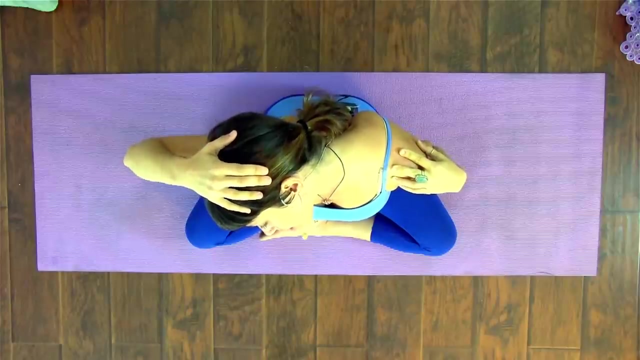 Reach your right hand up and over your right shoulder to the outside of your head, then bring your left hand to your left shoulder. now gently pull your hands apart, creating a little traction and adding to this stretch, and slowly begin to roll your chin down towards the floor. it's almost. 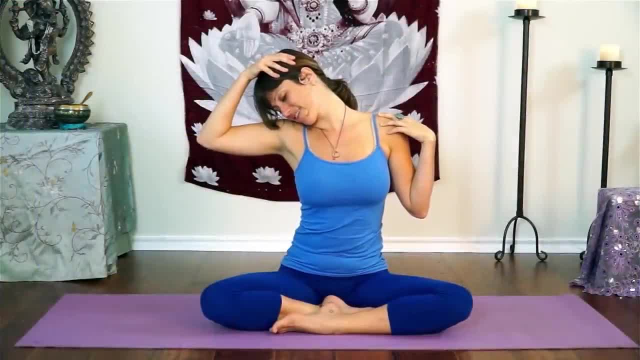 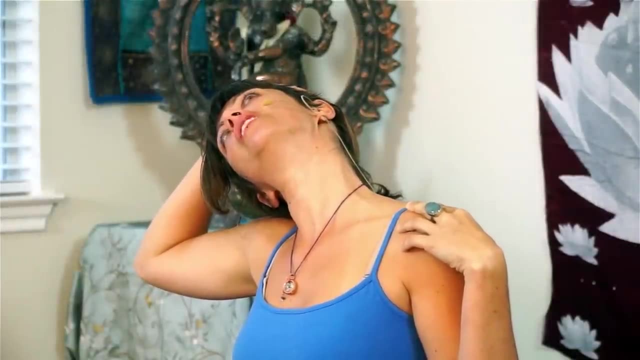 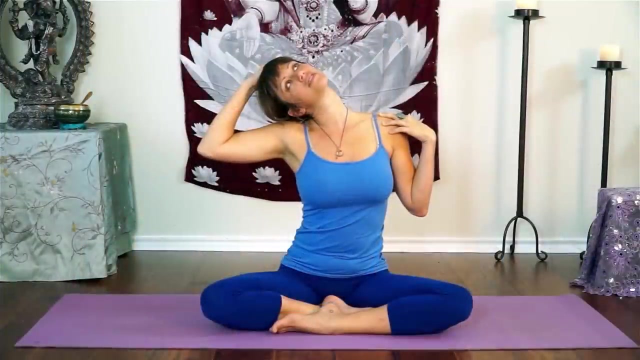 as if you are gonna sniff your armpit, which of course you wouldn't go. then slowly start to turn your chin up towards the sky and just notice how this little movement changes the stretch so you feel it in some different places. come all the way back to the right side and slowly come up to 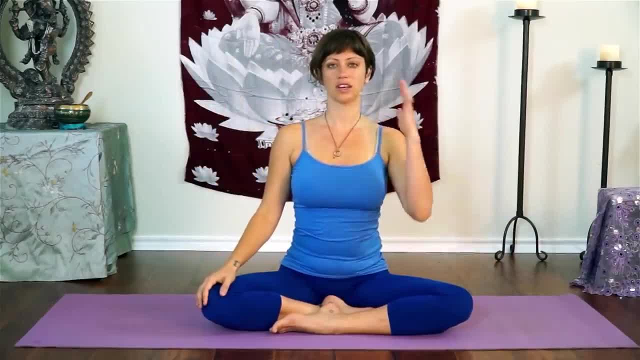 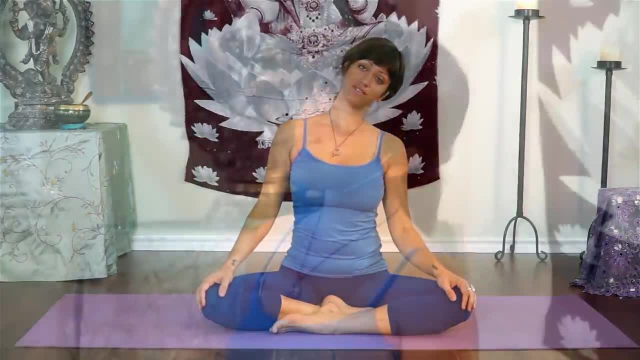 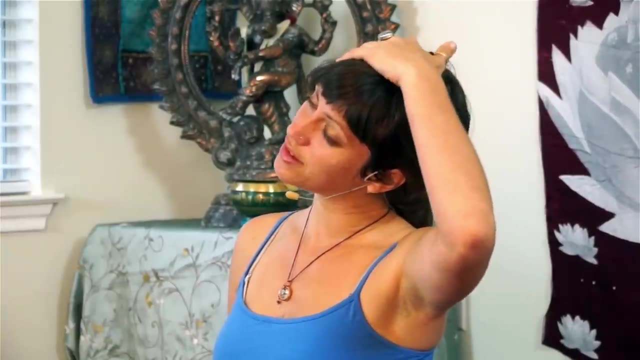 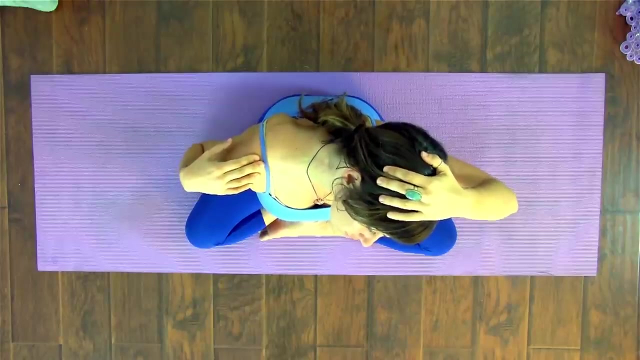 center. notice how that left side of your neck feels stretched and opened. then lower your left ear to your left shoulder and gently bring your hand up and over and your right hand to your right shoulder and apply a steady traction so you deepen the stretch along the right side of your neck. 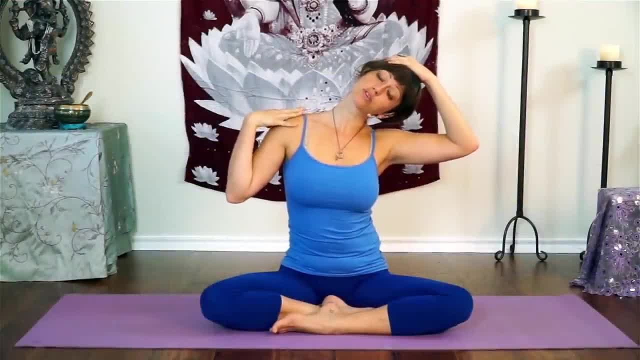 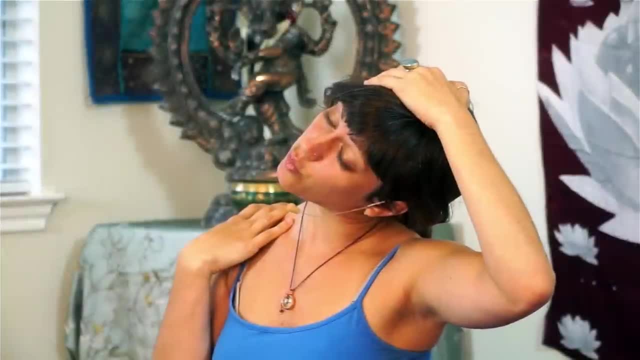 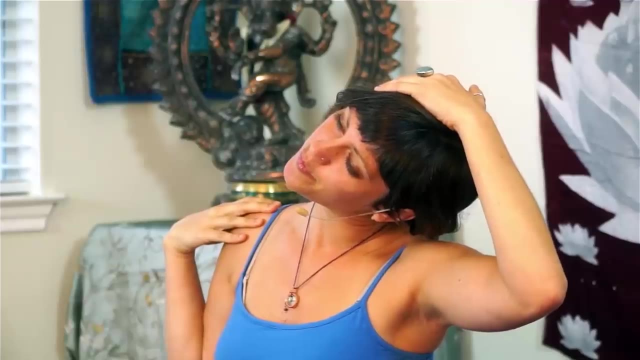 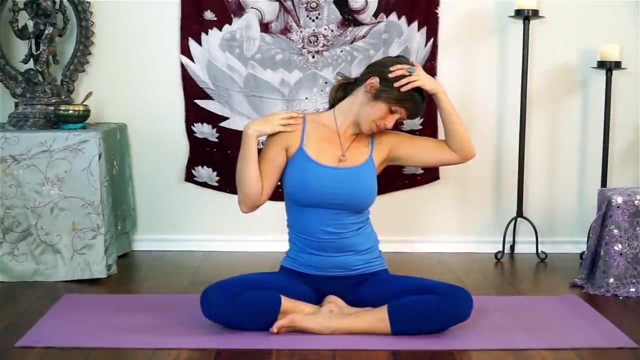 you and sometimes for people it's difficult to bring your hand here to the side. it may be easier to bring your hand in the front, and that can work as well. just want to have a little assistance to help you take this stretch deeper and roll your chin down towards the floor and slowly roll your chin up towards the. 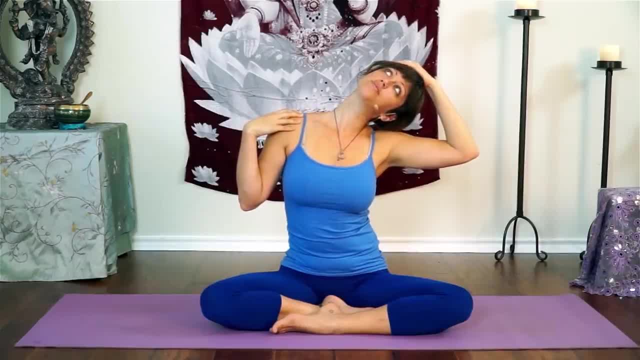 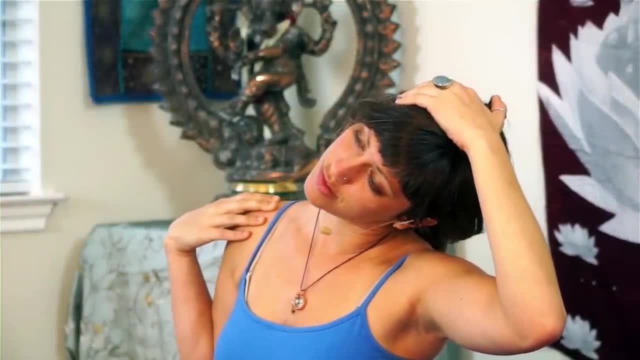 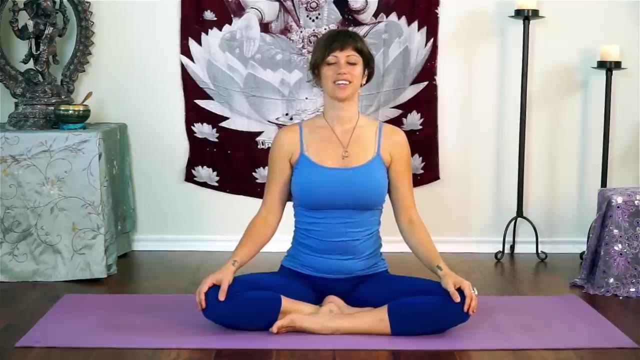 ceiling, the left foot over the right shoulder, right back and take another breath. go on and open it and we'll really clean up the now. we're gonna lay on a span, use the palm of your palm to turn around and bring your head to the ground while lifting your head up. so we're going to 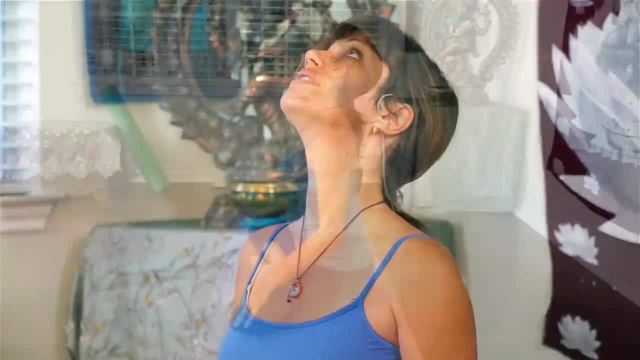 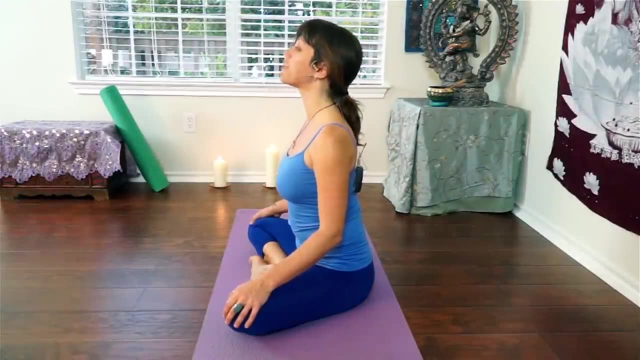 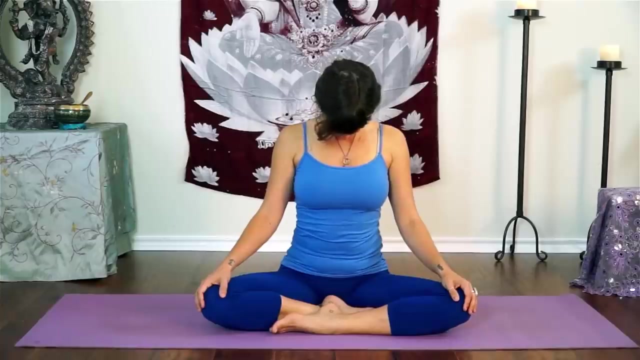 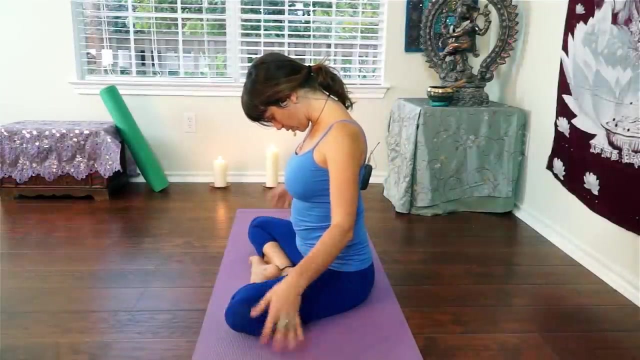 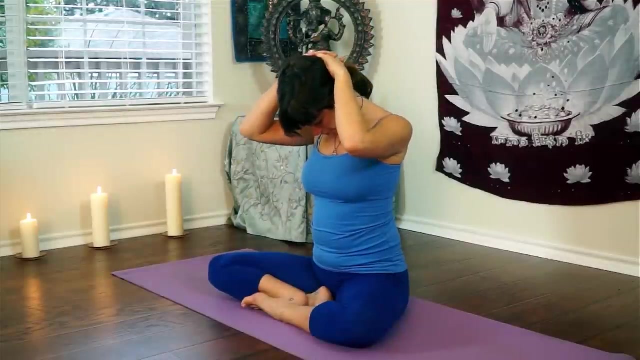 bring your head all the way up to the center, Looking down and up, working at your own pace according to what serves your body the most. This time, as you look down, pause here. then bring your hands behind your head, interlace your fingers, then let your elbows drop down towards the floor. 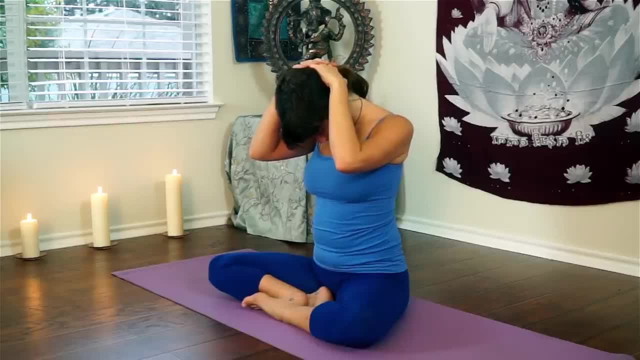 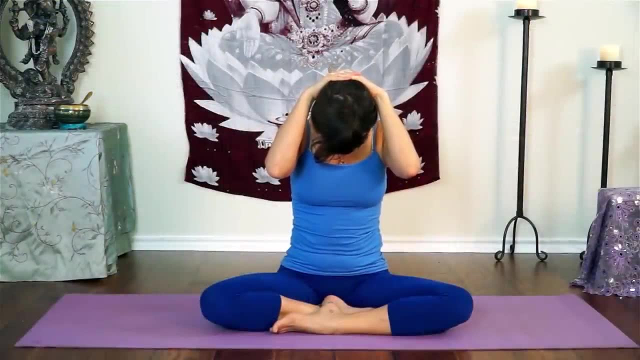 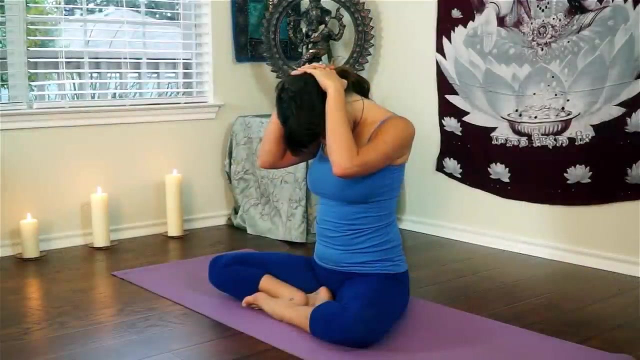 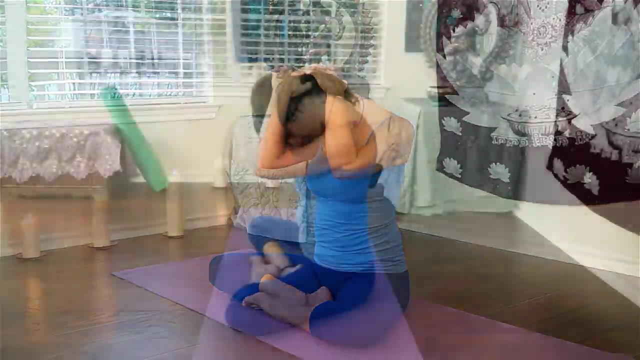 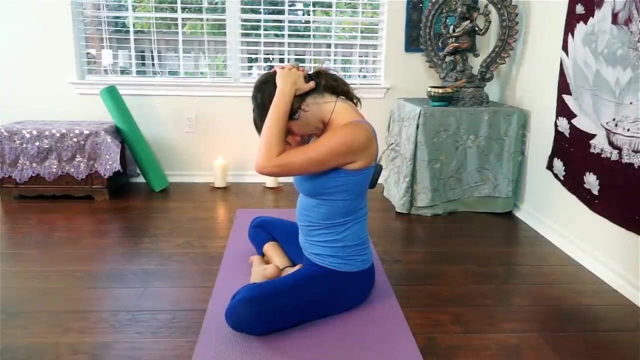 So now the weight of your arms will apply, that gentle traction along the back of your neck. Good, Don't forget your deep, steady breath. One more full breath in and a full breath out. Good, Good, And then throw the hands forward. 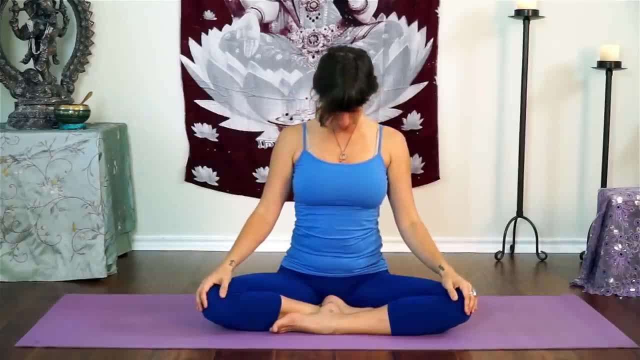 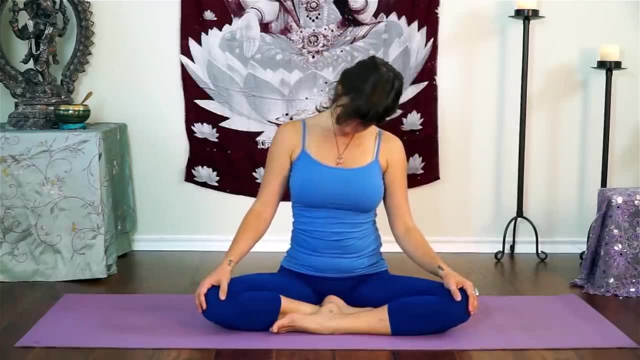 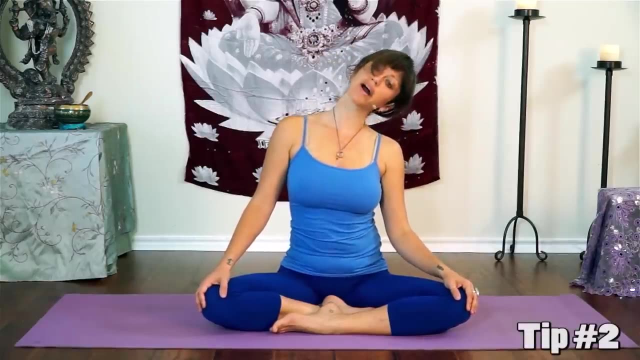 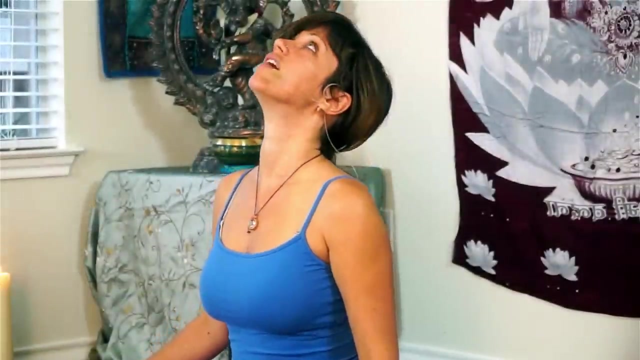 And then release your head and come all the way up to a seat. You can roll your head in a circle, going all the way around. And here I'll give you my second tip for reducing back pain is to move your body more. Our joints get stiff. 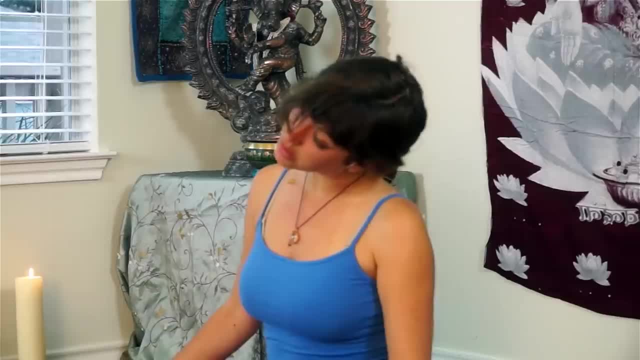 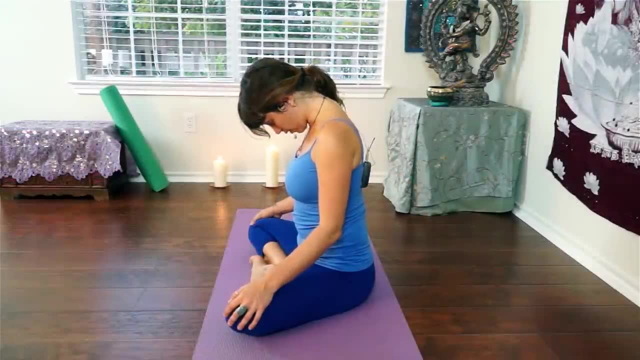 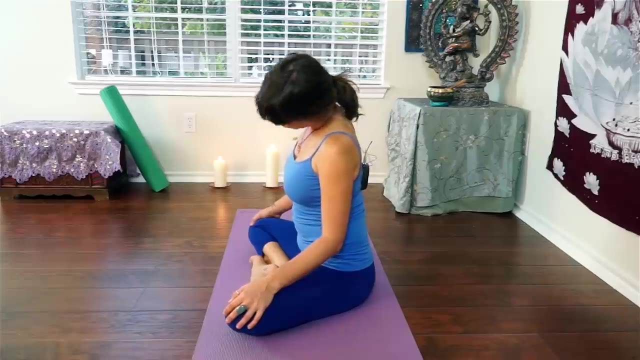 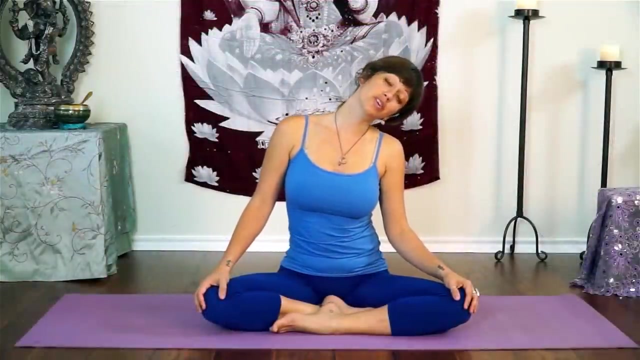 Yeah, and our muscles become weakened when we sit still all the time change directions of your circle. so if you remember the tin man from the wizard of oz, he was stuck in that standing position for so long. when they finally found him, it was hard for him to move his joints. and that's how it is with our bodies: when we don't move, we become stiff. 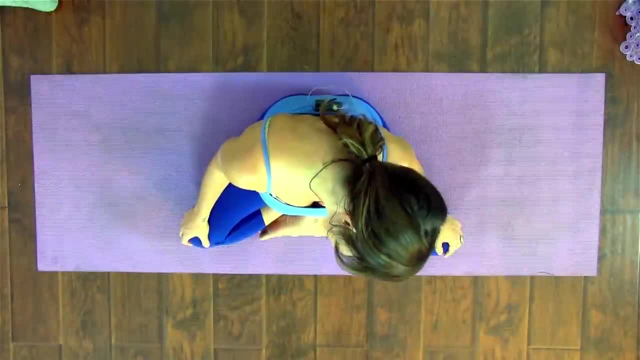 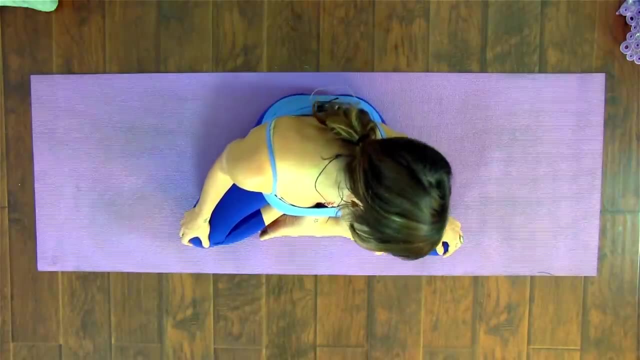 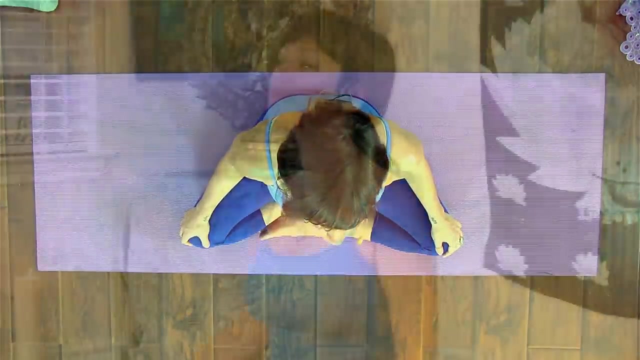 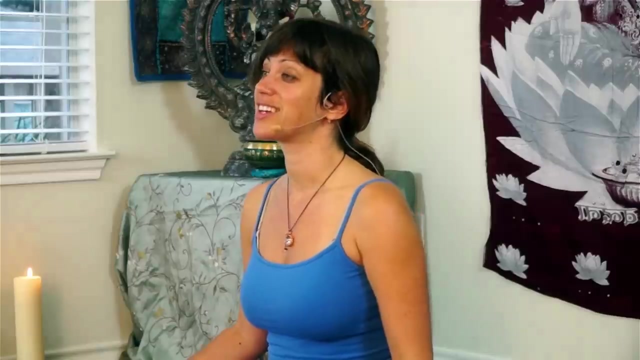 and achy. so whatever you do, even if it's just these simple head and neck stretches or taking a walk, getting up and walking around the office, bring your head back to center. any kind of movement you can include it's going to help your body keep limber and strong. 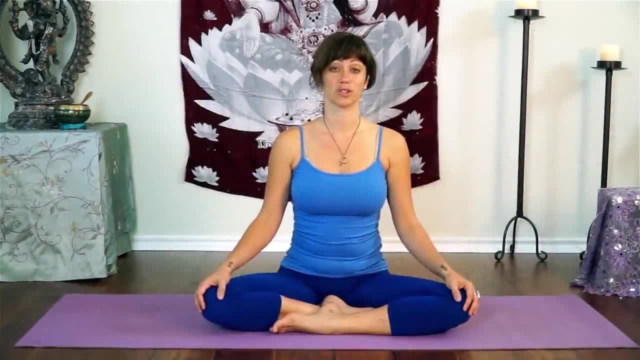 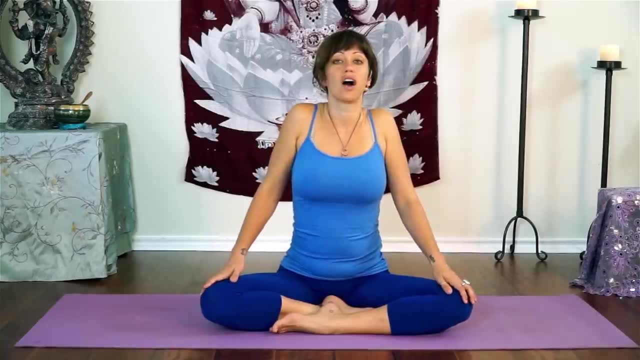 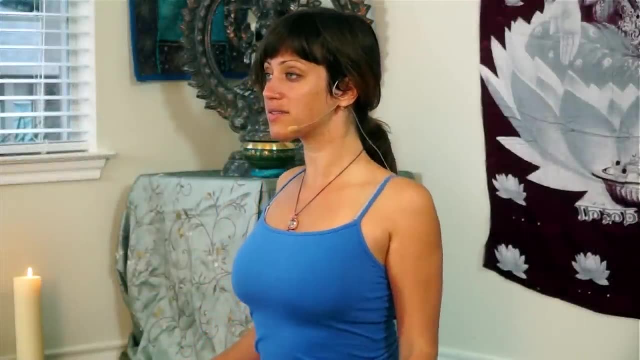 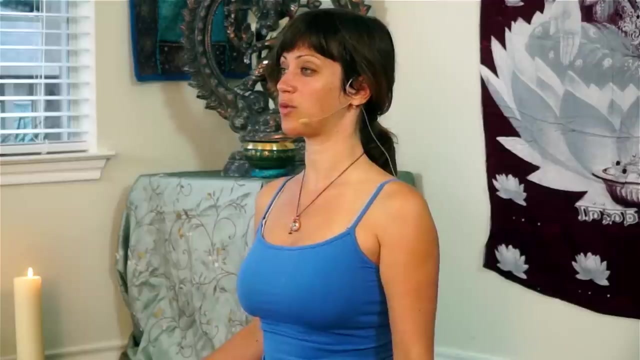 let's move down into our shoulders, start to roll your shoulders back and, as you do, hug your shoulder blades together and spread your chest wide. rolling your shoulders back, let's reverse directions and we're going to start to move our shoulders back, so this time we roll to the back, up and forward. 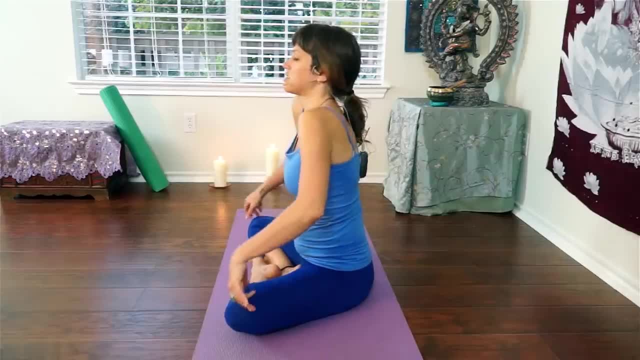 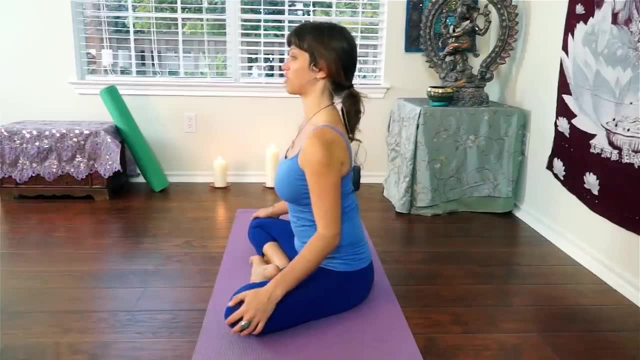 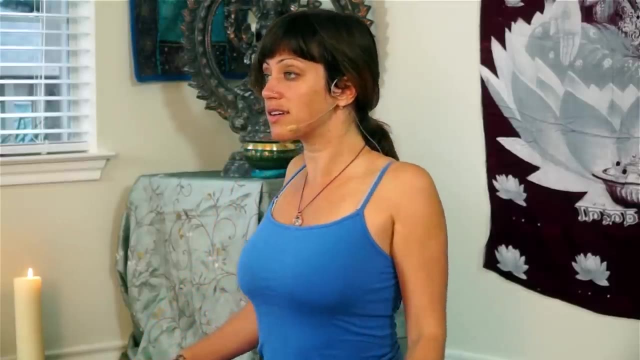 so let's just really think about your shoulder blades. you want to get those shoulder blades moving as much as you can. let's reverse directions again, going to the back, feel your shoulder blades squeeze closer to your spine and move farther apart as you make these big circles with your shoulders. 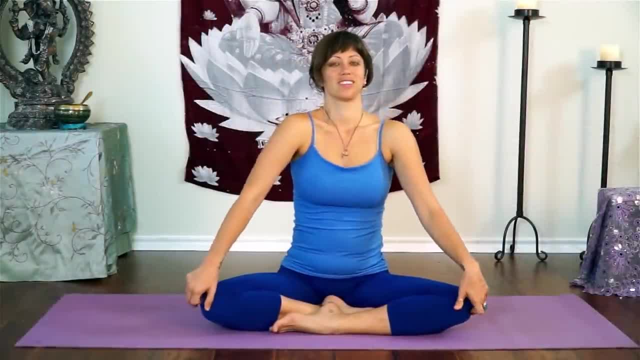 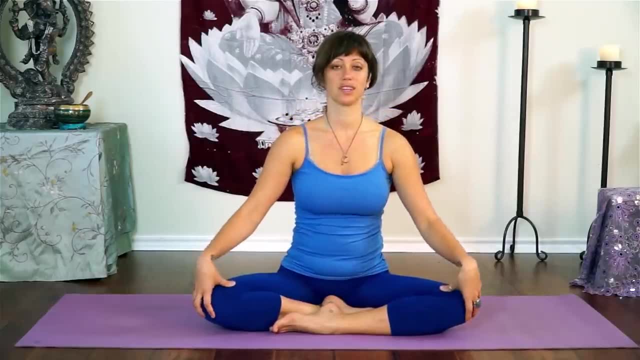 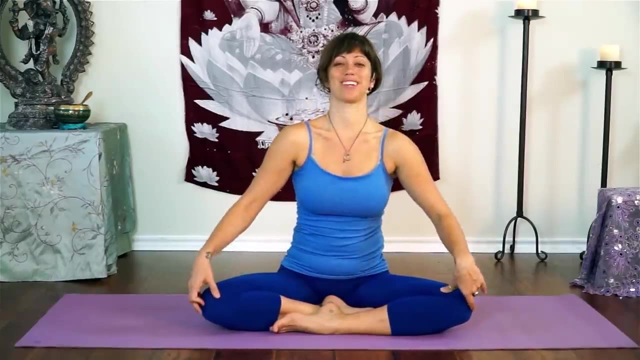 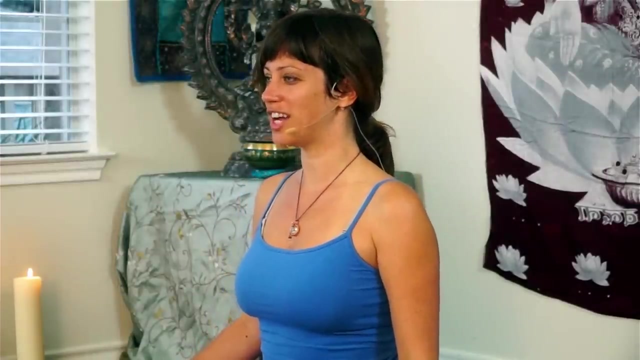 let's go forward one more time. this is also going to build a little bit of strength in your traps and your upper back muscles, so they get tired and weak from sitting, and so this is going to help wake them up and get them strong. all right, so now we're going to move into a side body stretch. 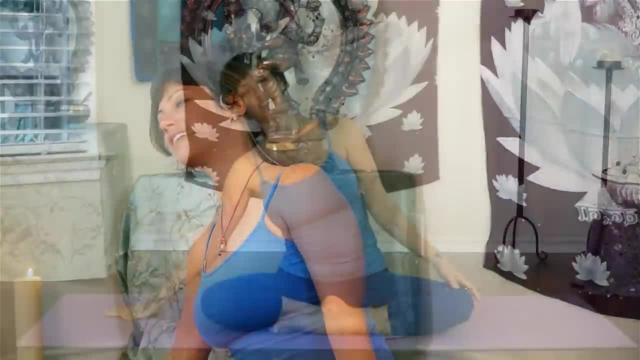 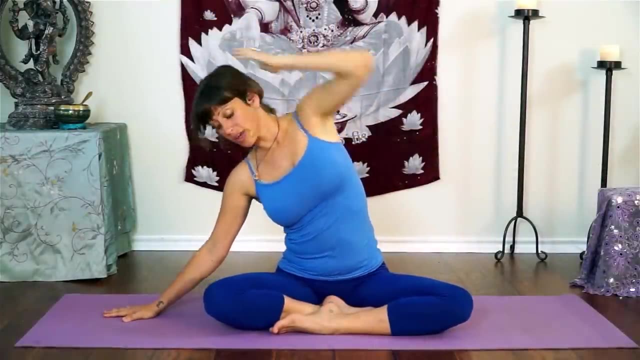 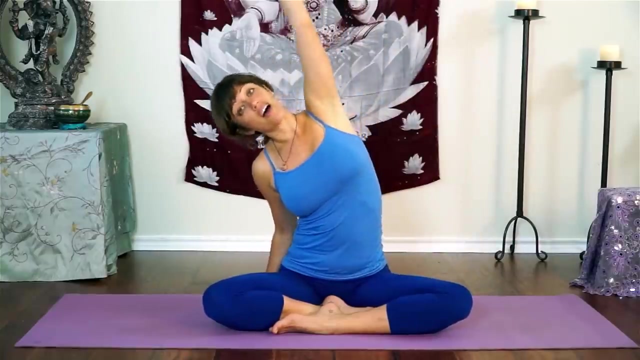 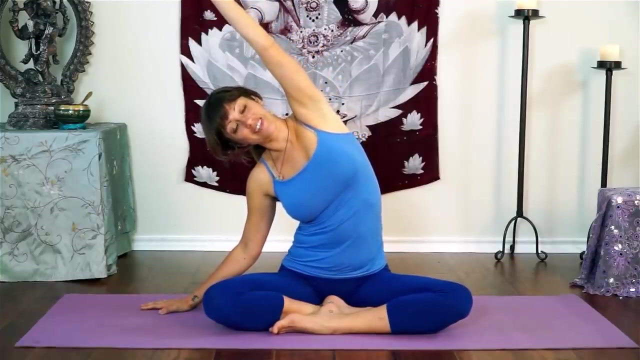 so reach your right hand way over to the right and reach your left arm up and over. if you're sitting in a chair, you can bring your hand down onto the seat of your chair to give you some support while you lean up and over. so, wherever you are, however you're seated, think about your left hip bone. 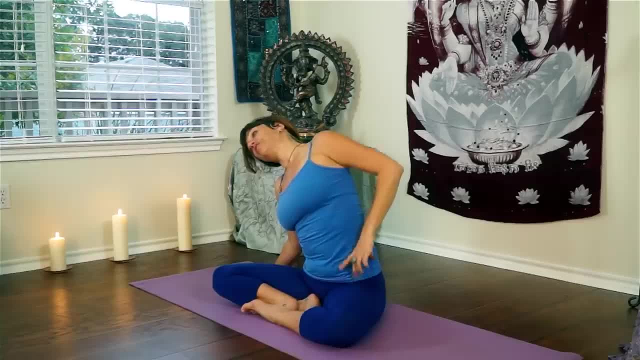 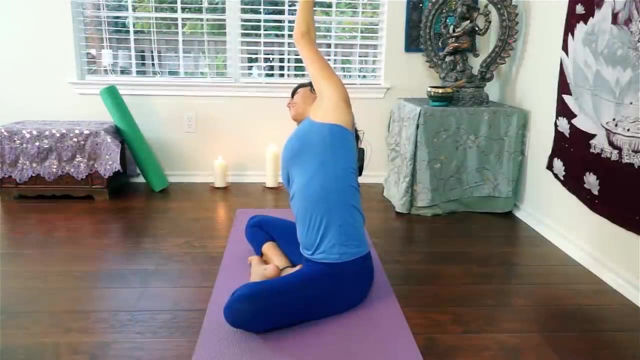 grounding down towards the earth. so this is your anchor. then stretch with your left arm, reach all the way through your left fingertips so that the entire left side of your body is activated and stretching, lengthening. you should feel some sensation here. and let's come all the way up. 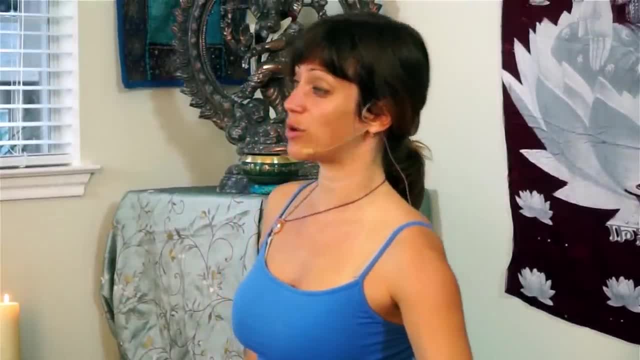 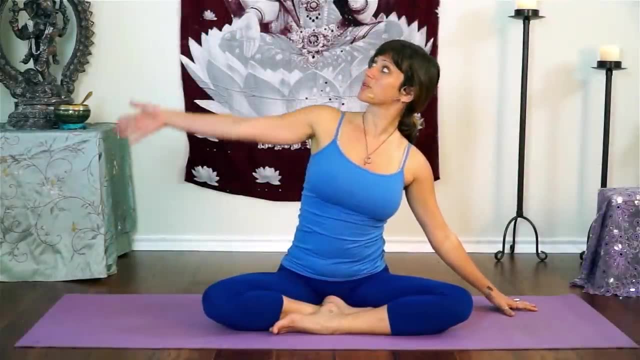 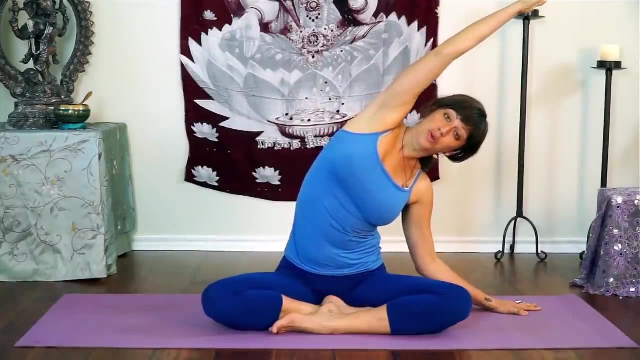 and switch sides. so bring your left hand over to the left or onto the edge of your seat. if you're sitting in a chair, then reach your right arm up and over at the same time that you ground down with your right hip. reach all the way through your fingertips so that even your elbow is straight. 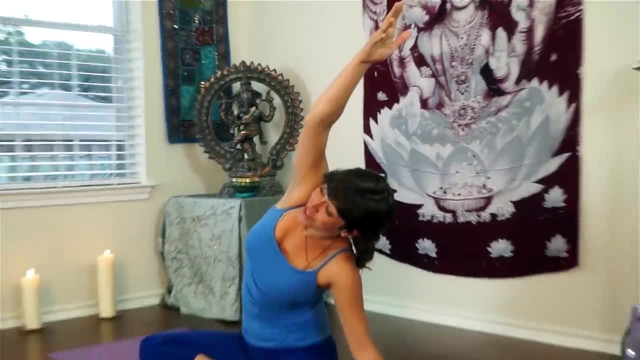 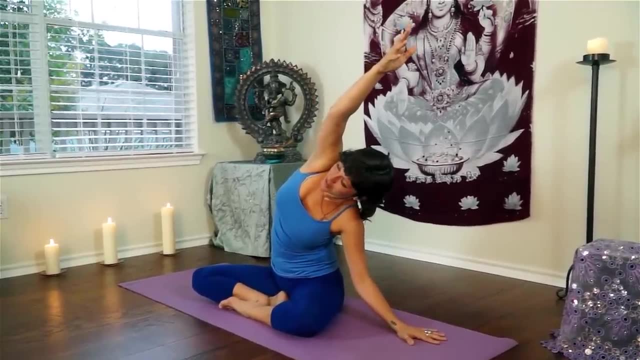 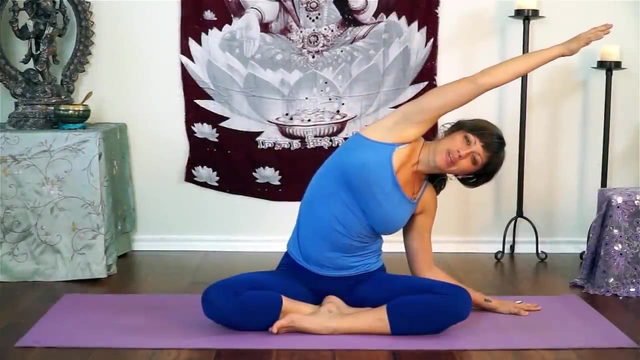 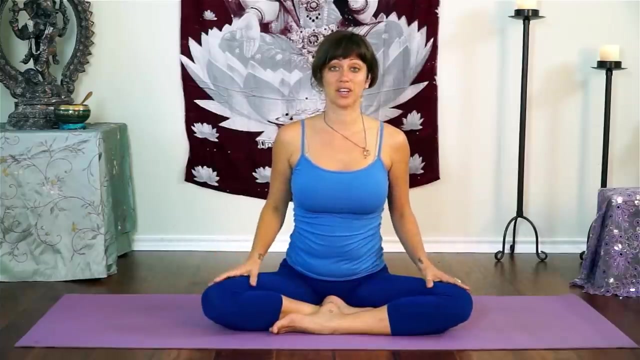 that's going to intensify the stretch and that's good. so you really want to get into it, don't be scared. creating a nice opening along the right side of your body. reach as far as you can and we'll come all the way back up and we're going to get into a little movement again here. i call this a full body swoop. 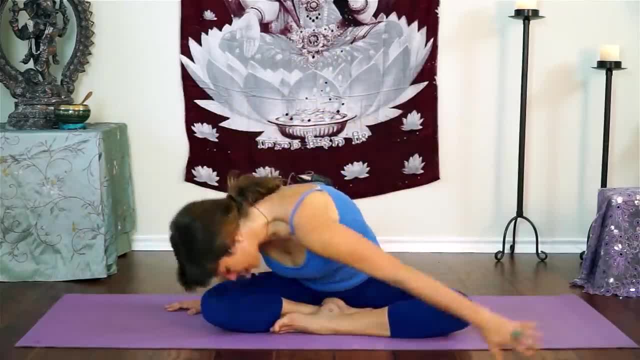 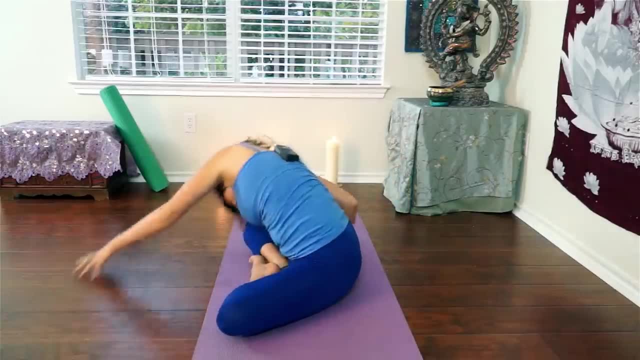 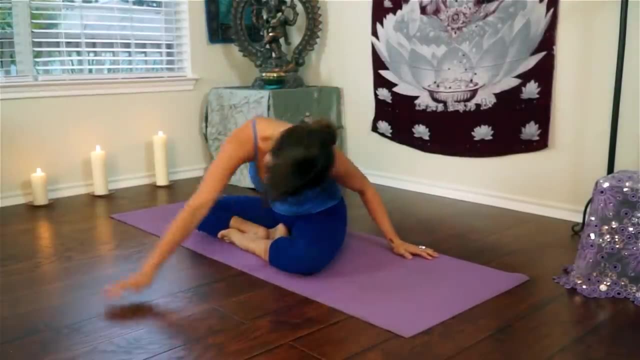 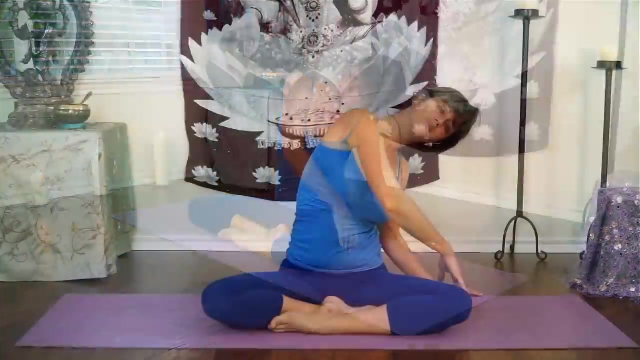 you're going to start to the right side and just swing your body, your torso, through the center and come to the left and just sweep around from side to side. be nice and gentle with yourself. no need to get crazy, but just allow that movement to reverberate through your spine and stretch all those muscles that get tight and tired. 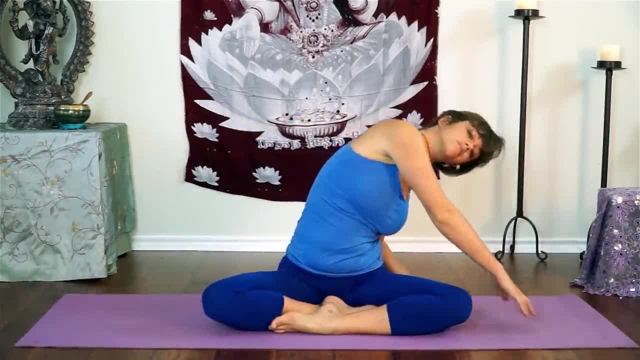 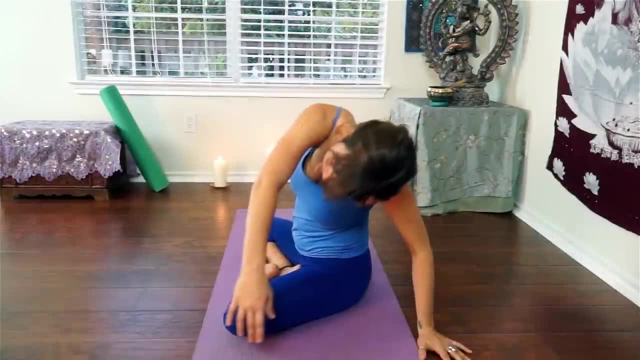 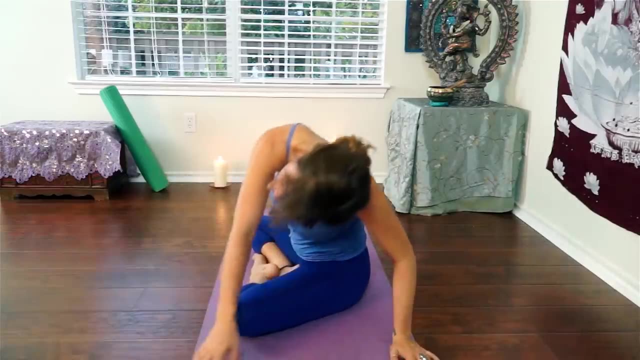 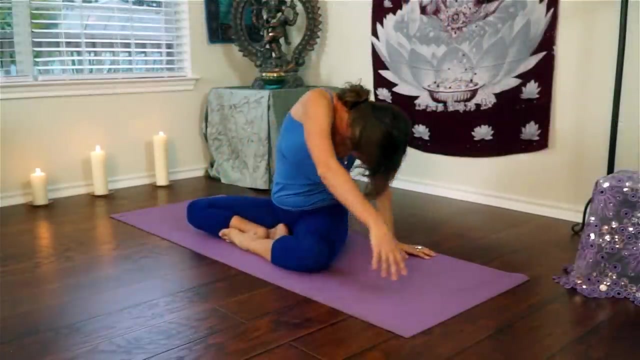 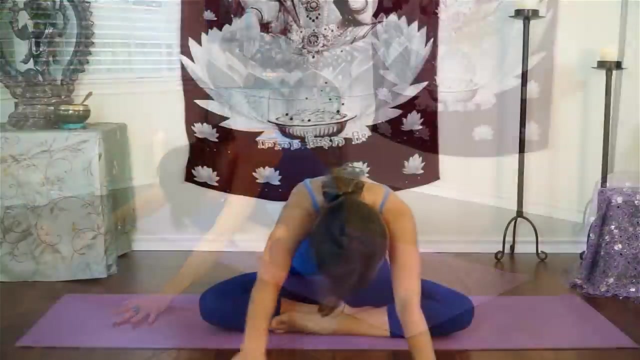 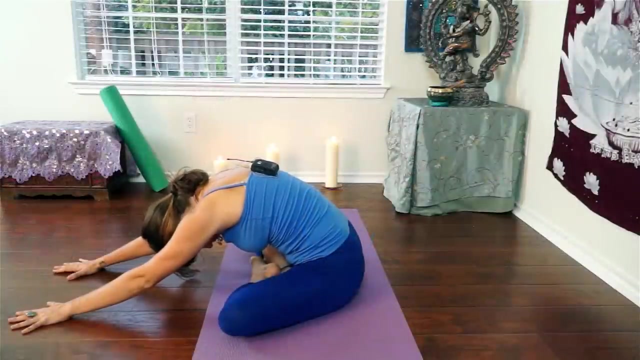 and your legs will be good for a little bit as well. so again you're moving at your own pace. take your time and just enjoy the movement. so again you're moving at your own pace. and then come to center. just stretch your body forward, you will probably feel. 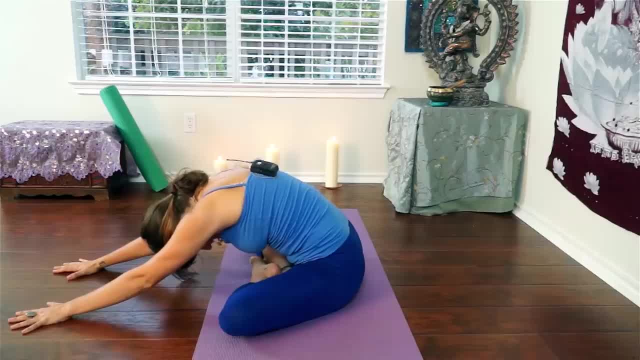 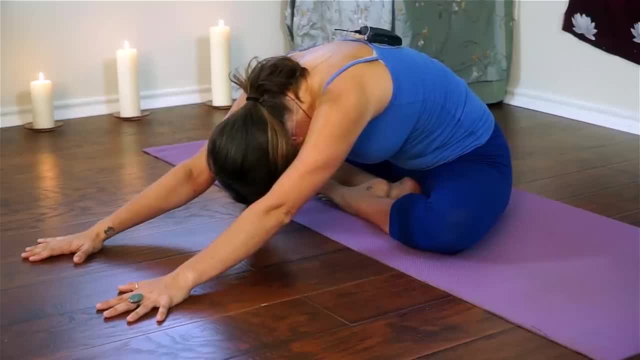 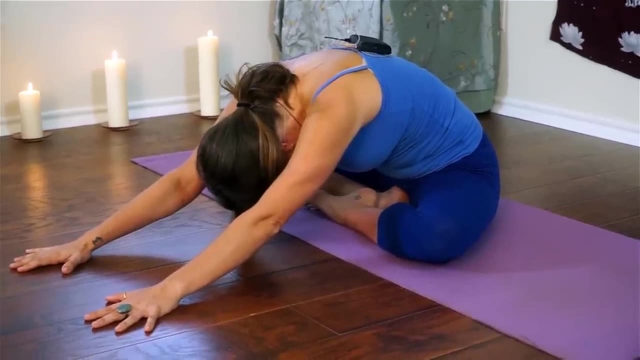 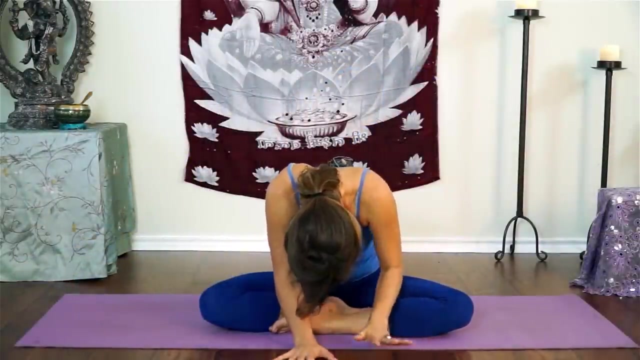 a little stretch in your hips. that's a good thing. our hips get really tight, so a little stretch is nice. we're gonna start coming back up to a seated position now, but I want you to go really slow and think about stacking your vertebrae one on. 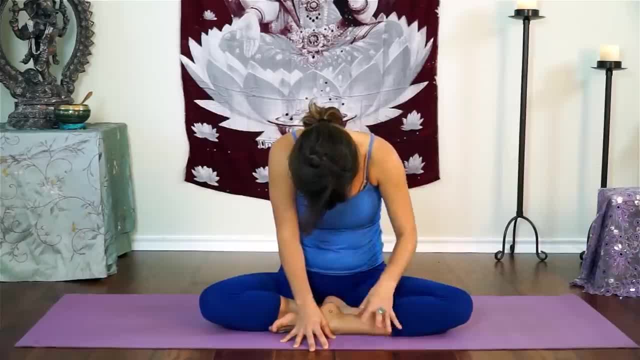 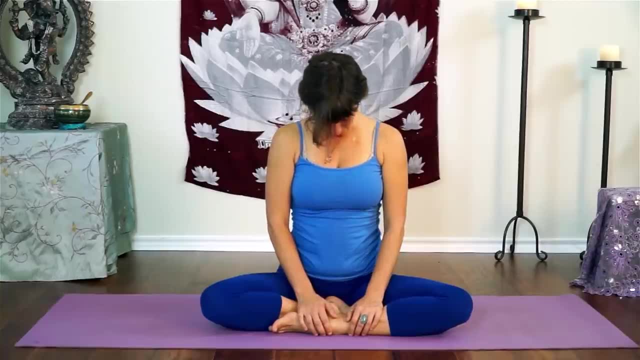 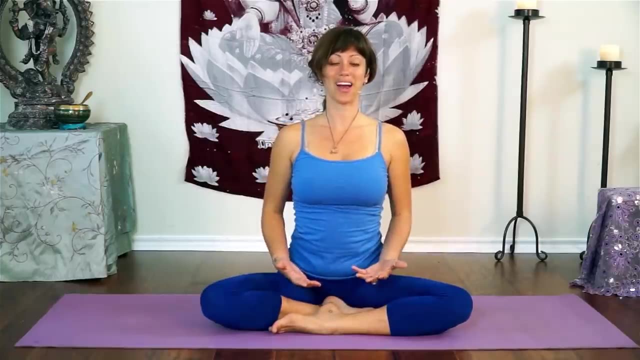 top of the other. so you go slow. your head will be the very last thing that comes up as you unroll your spine. and when you come all the way up, right, you'll notice that your spine is a little bit higher than your head. and then you come all the way up. 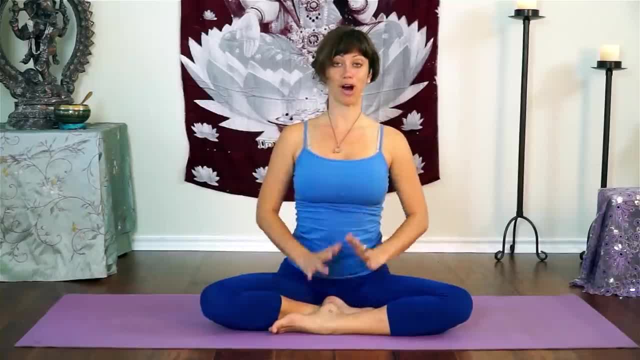 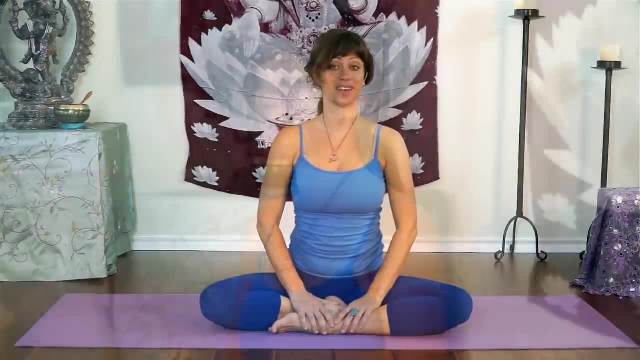 you'll notice that your spine is a little bit higher than your head, and then you come all the way up, that you're in a really great, healthy posture. and that brings me to my third tip for reducing your back pain is to think about your posture. remember when 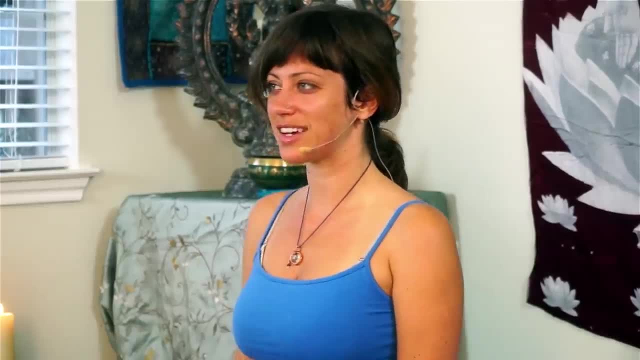 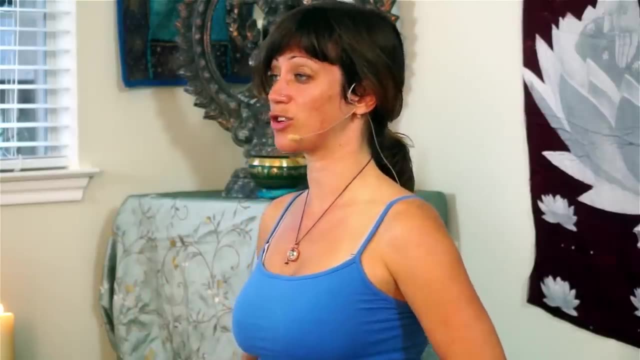 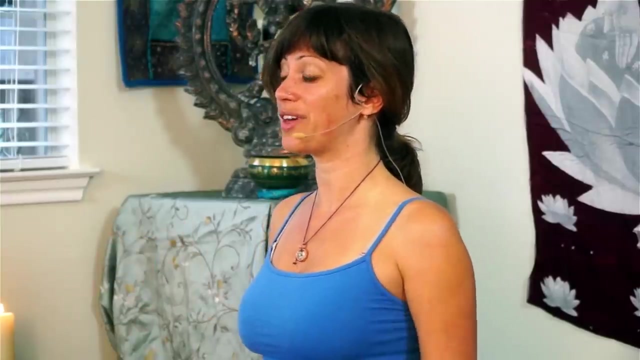 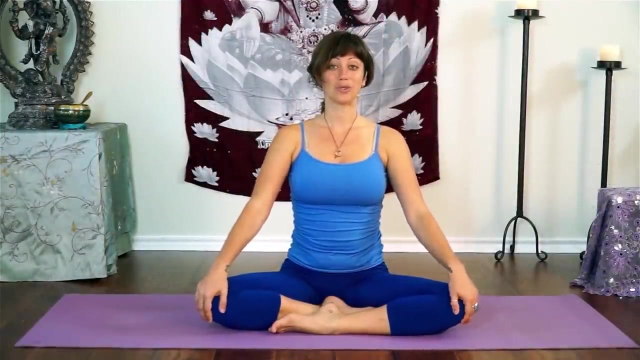 your back starts hurting and things get stiff. sitting upright, mindfully, is gonna help build the strength of your deep core muscles and help you to reduce your back pain by having a healthy and supportive posture. so from here we are going to do a little cat and cow seated, so you're gonna start. 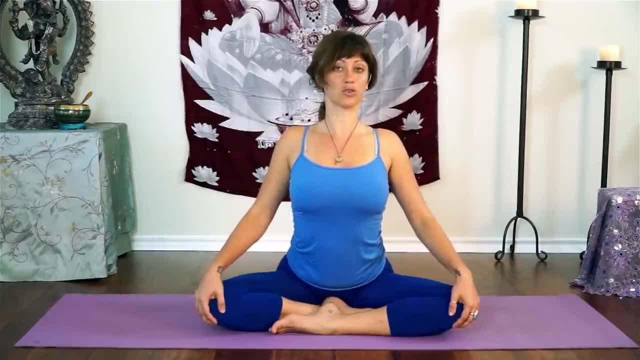 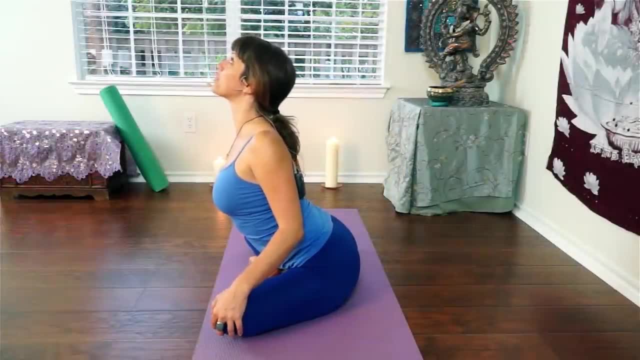 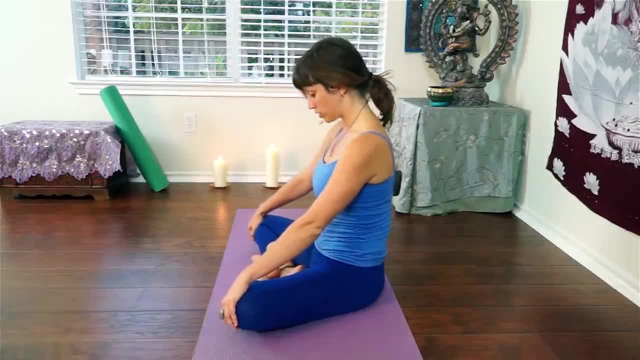 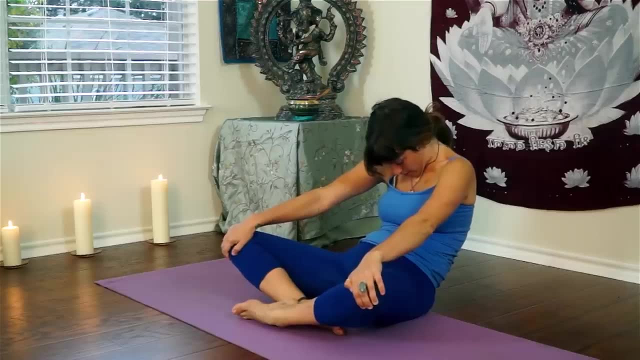 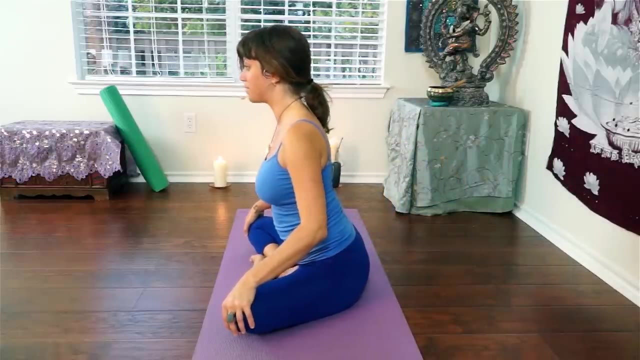 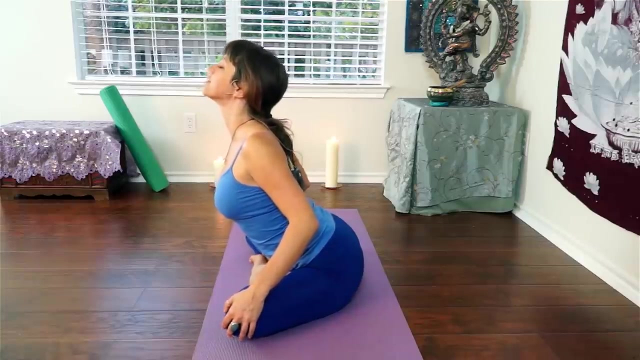 round your spine, tuck your chin into your chest and rock back on your sacrum so you stretch your spine. then come forward again, take an inhale here, a big breath in, and, as you start to round your spine, exhale. and as you start to round your spine, exhale. 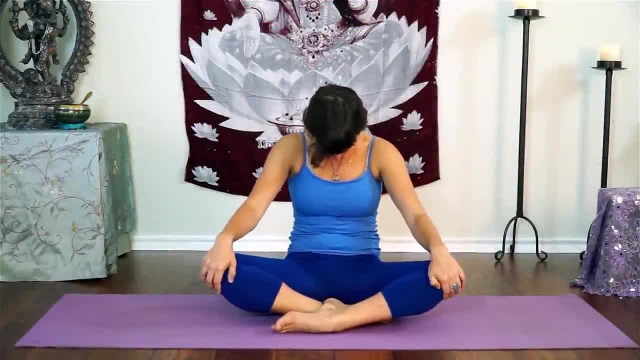 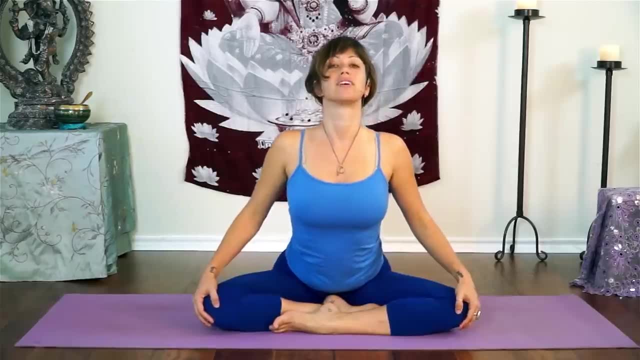 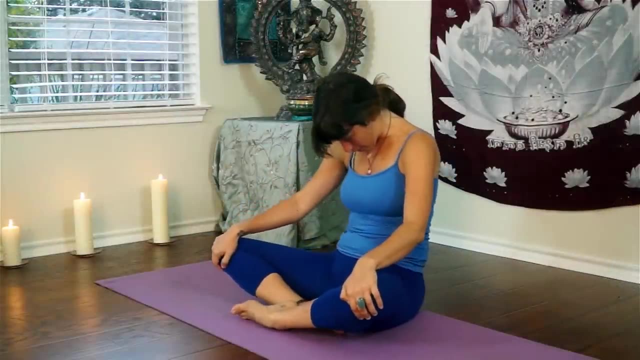 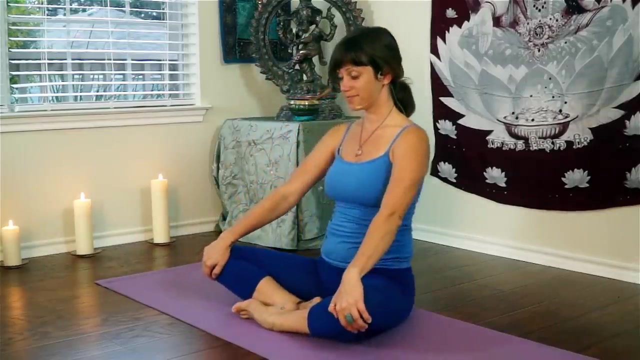 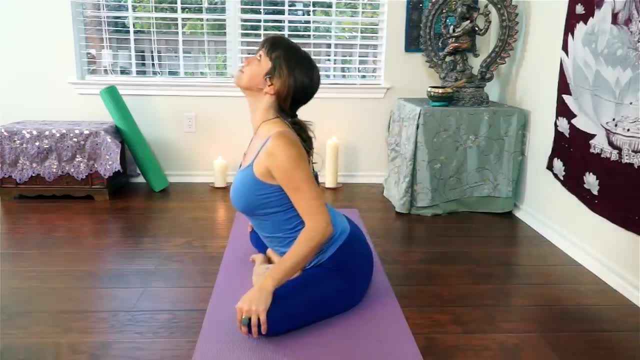 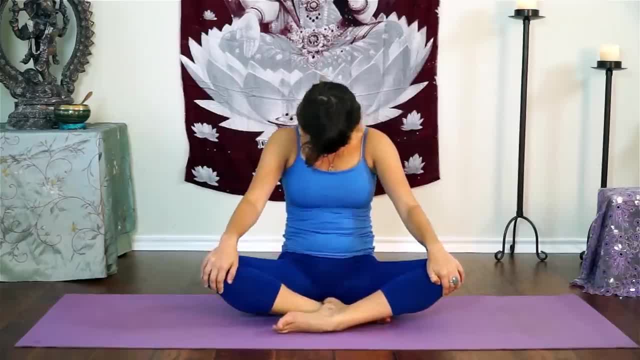 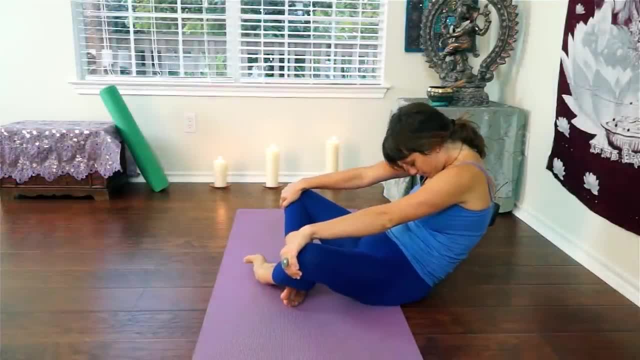 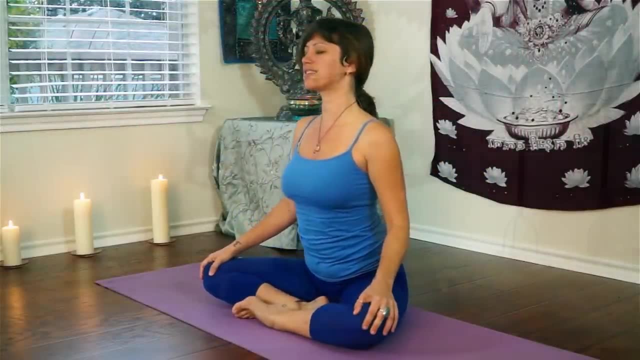 so again you can move at your own pace. honor the rhythm of your own breath. so again you can move at your own pace, honor the rhythm of your own breath. Then come all the way back up, stacking your spine, stack your vertebra, nicely, so you. 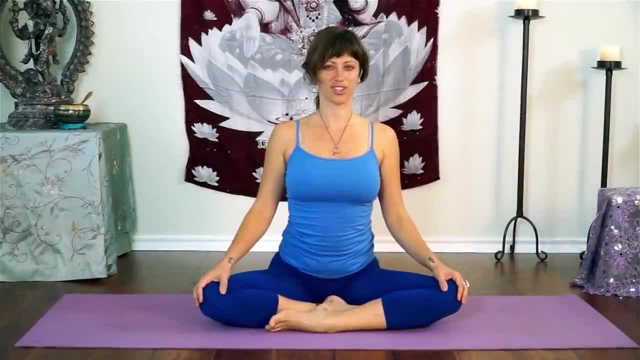 come all the way up into that healthy and supported posture. The more you can practice this upright alignment, the more you're going to build a muscle memory and build the strength of these muscles. so it's going to get easier all the time. Let's take a twist. 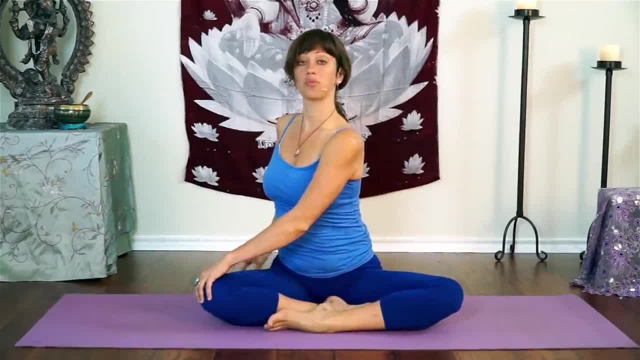 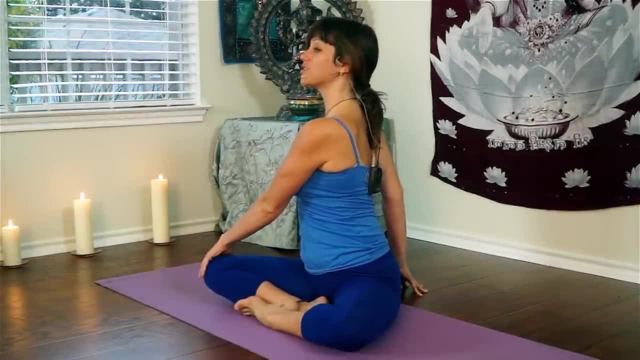 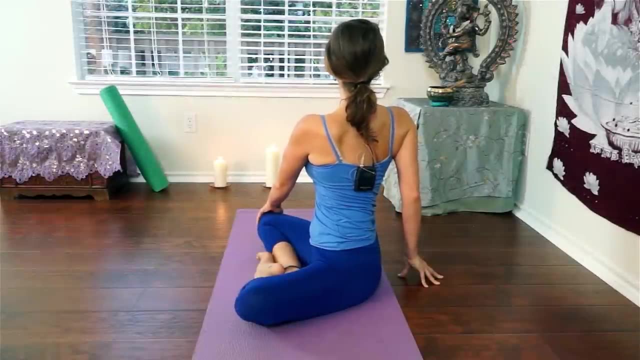 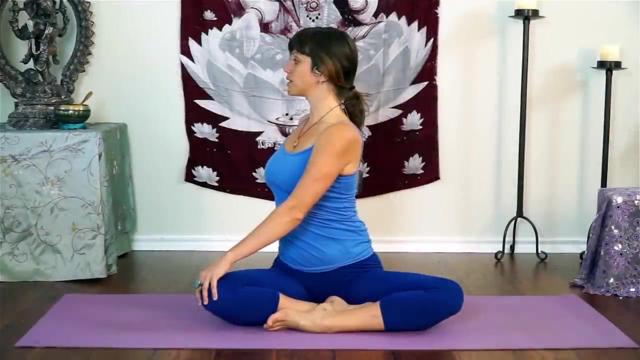 Reach your left hand across to your right knee and bring your right fingertips behind you. Lift up on your spine, sit up nice and tall. then twist your heart towards the right. Use your arms to give you some traction, to help you get deeper into this twist. 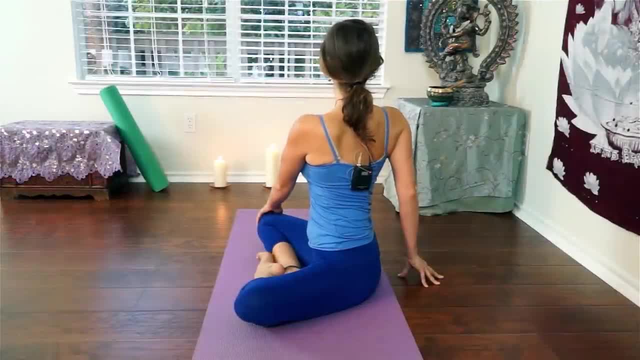 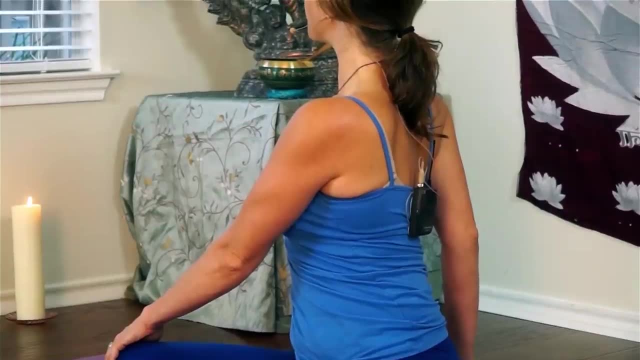 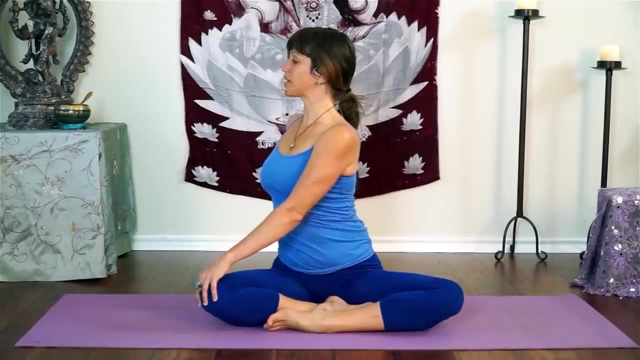 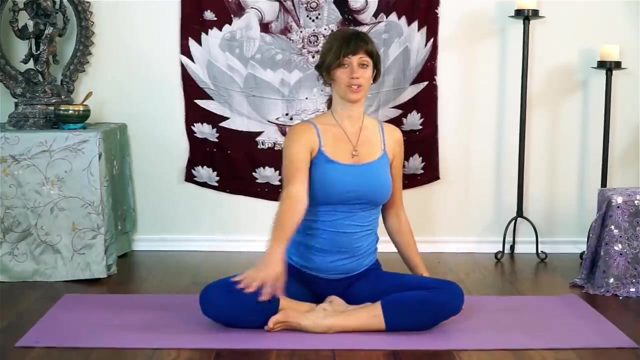 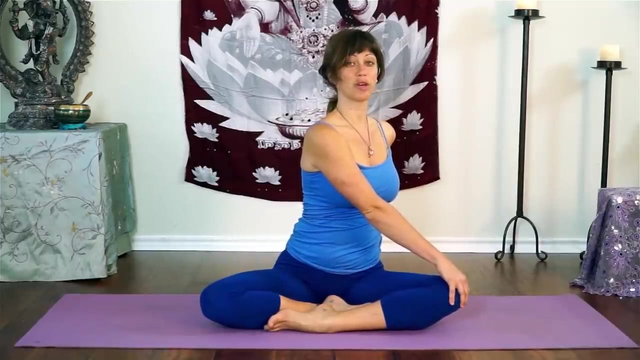 Keep sitting up, Keep tall and keep breathing deeply. Make your way back to center and let's move to the other side. Reach your right hand across to your left knee, Bring your left hand behind you, Take a big breath in as you sit up, nice and tall, and as you exhale, twist your heart. 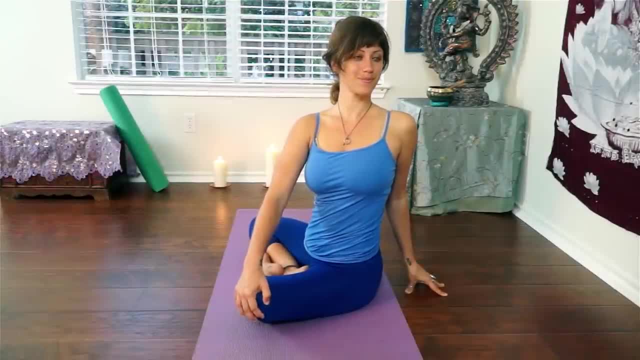 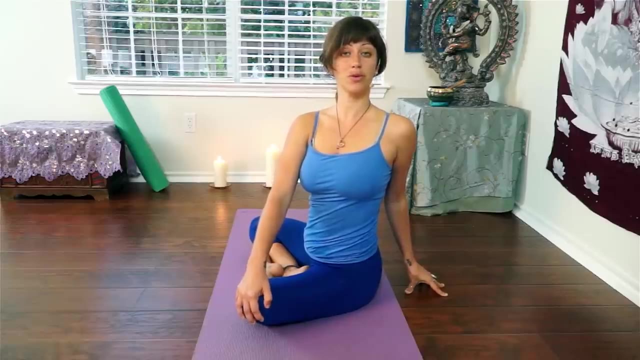 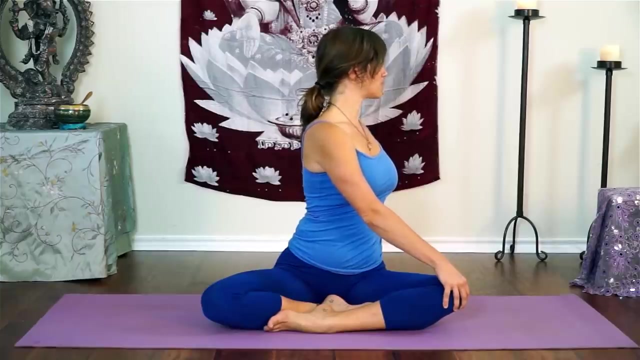 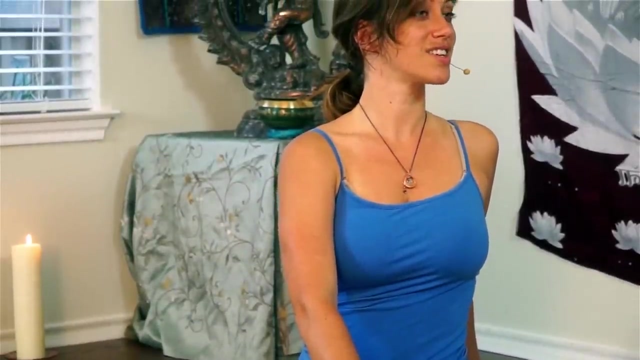 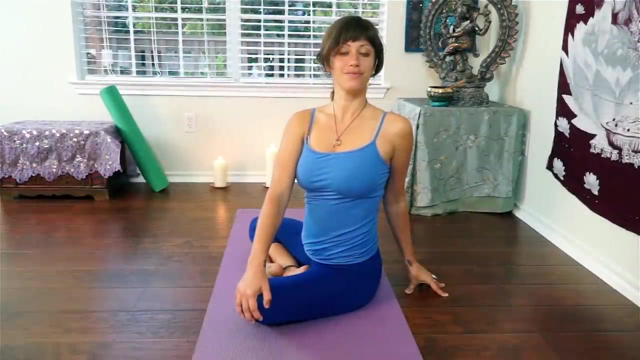 towards the left. The more you can sit up straight, the more space you'll have in between your vertebrae to twist even more. Of course you don't want to force anything. Don't go beyond what's comfortable for your body, but find the edge, your maximum twist. 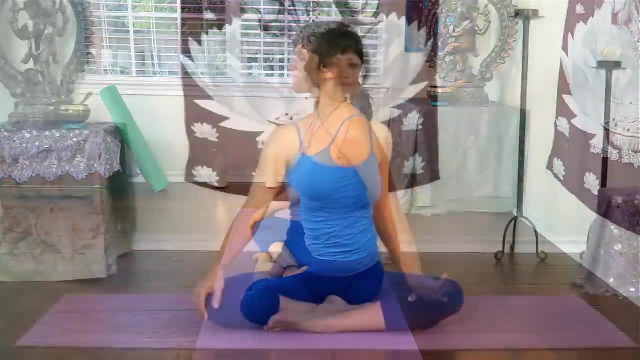 Then come back to center And from here we're going to move on to our hands and knees, And from here we're going to move on to our hands and knees, And from here we're going to move on to our hands and knees. 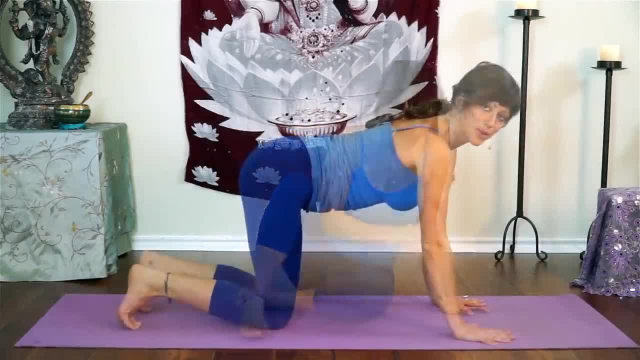 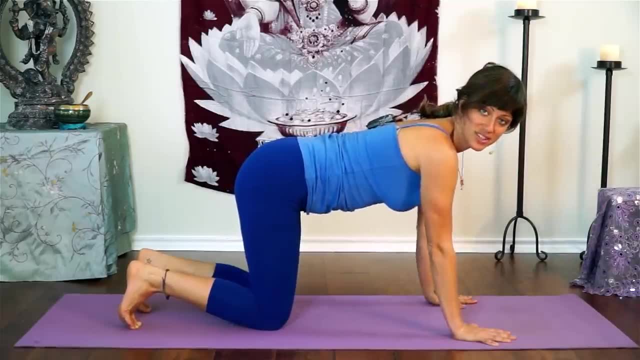 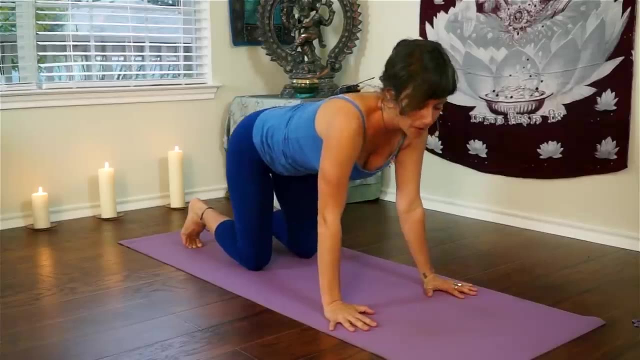 So you'll come into a tabletop position. So in your tabletop, make sure that your shoulders stack directly over your wrists and your hips stack directly over your knees. Then we'll take this cat and cow again. So, just like when we were sitting down on your inhale, lift your chest and lift your. 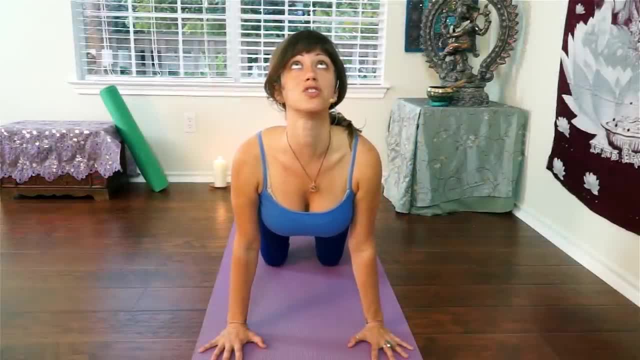 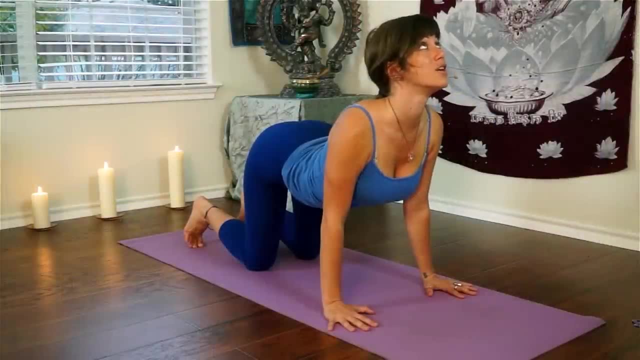 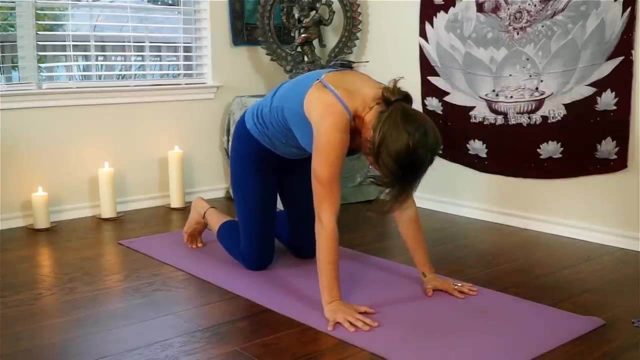 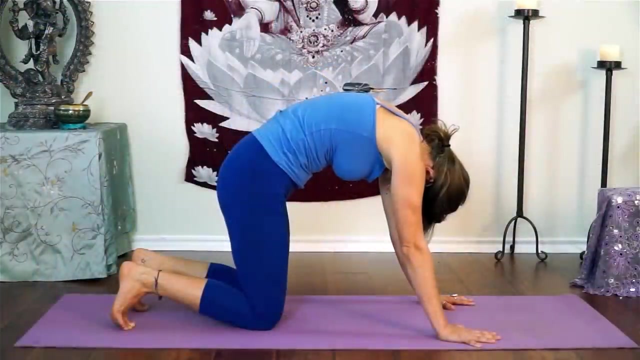 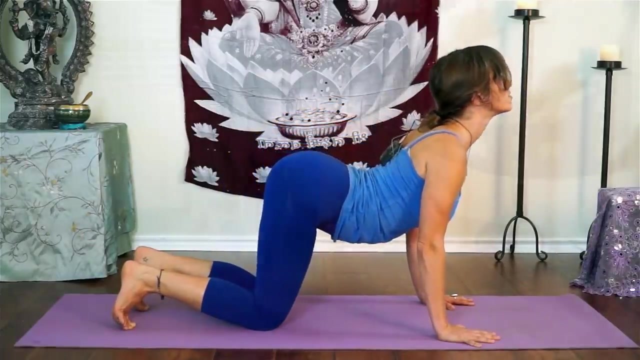 tailbone. squeeze your shoulder blades towards your spine and open your throat. then, as you exhale, round your spine by tucking your chin to your chest. press your hands into the floor to help you. stretch your spine up towards the ceiling. inhale to lift your head and your tailbone towards the sky. spread your collarbones apart. 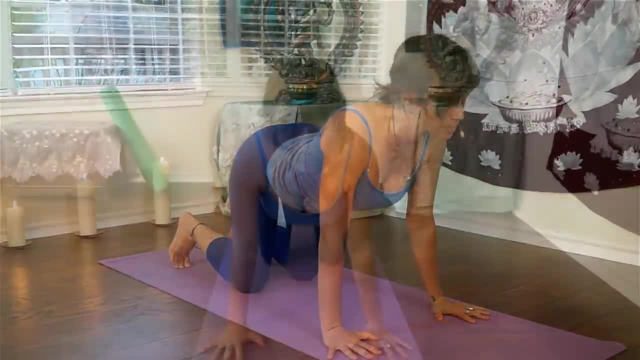 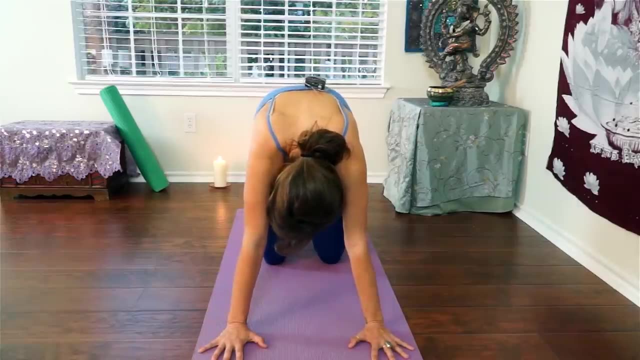 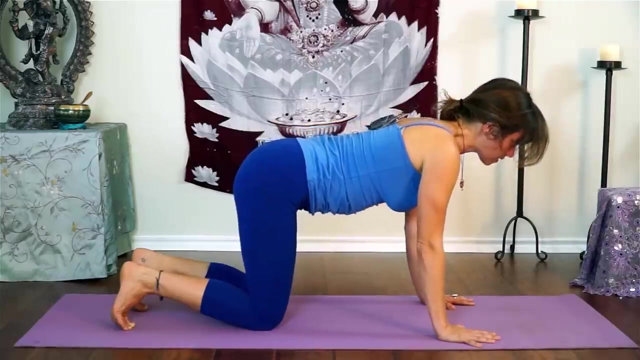 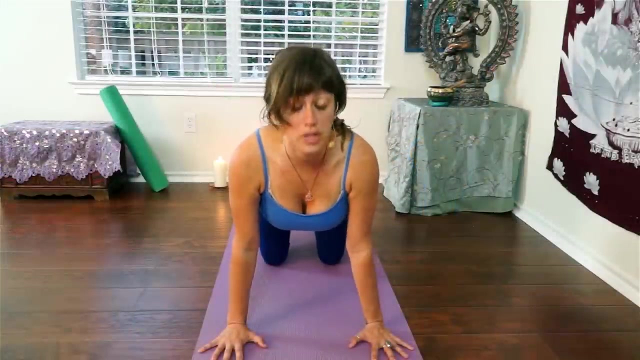 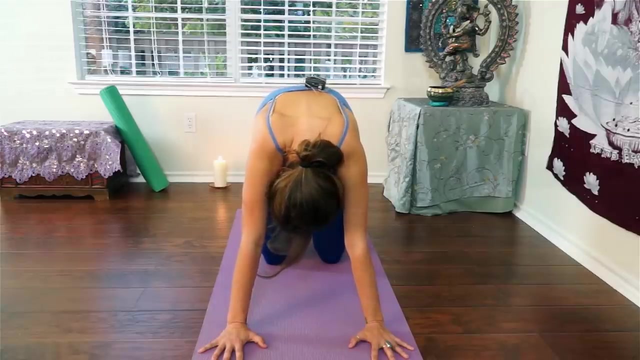 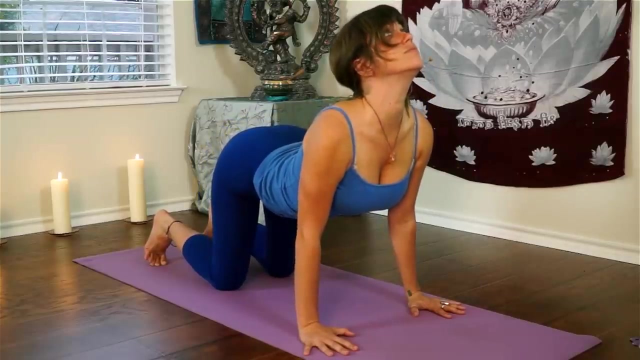 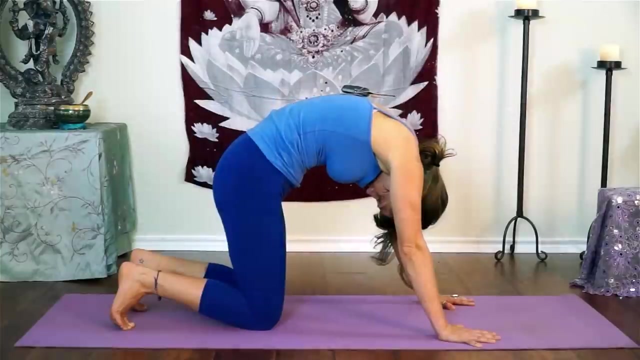 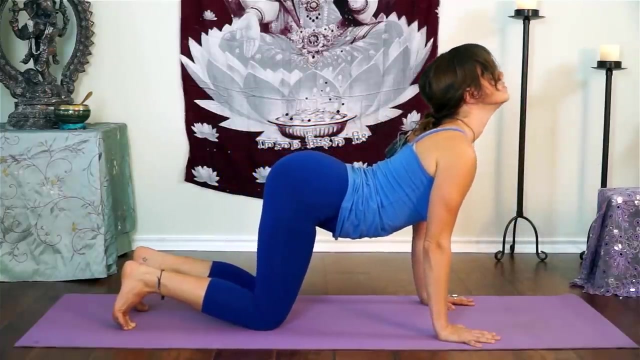 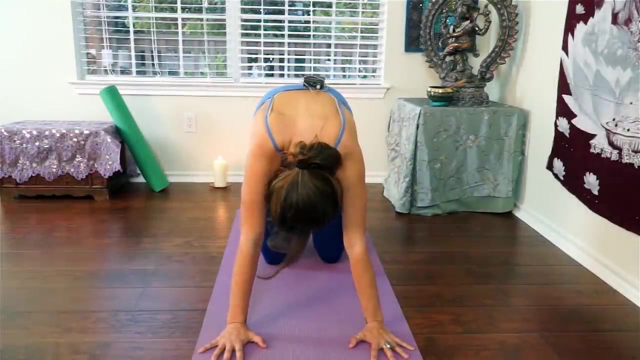 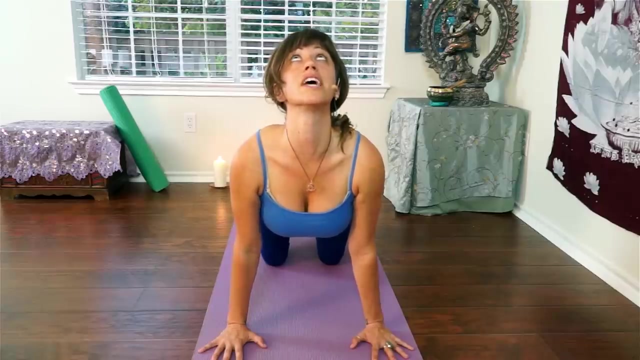 then exhale and round your spine, press the floor away so you get a nice stretch along the back of your spine. so we'll take this a few more times. move with the of your own breath as you inhale to open and exhale to close. we'll finish up with one more round: full inhale and full exhale. 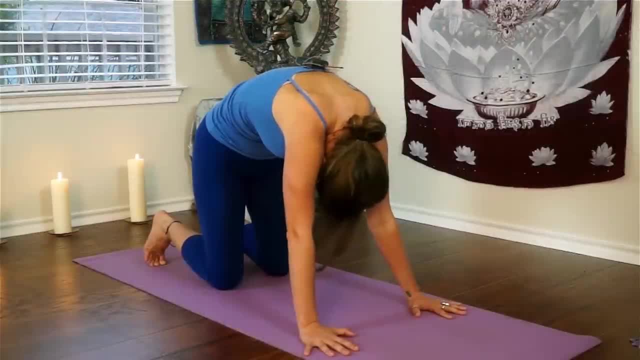 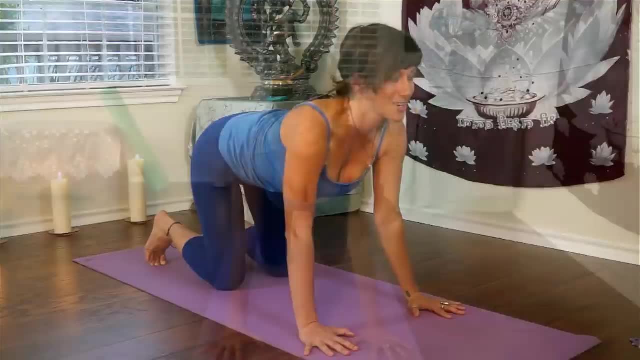 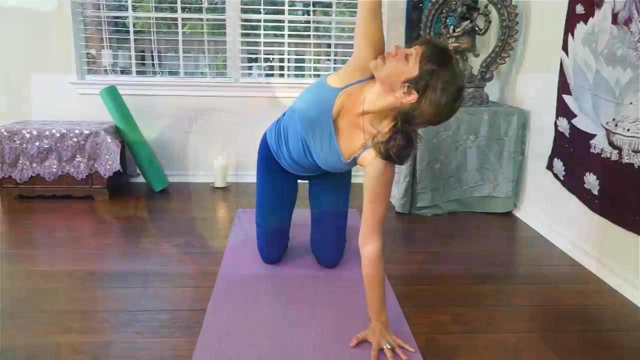 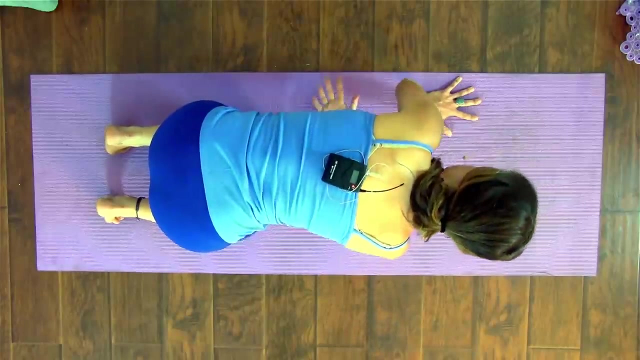 and we'll come back to center. so we're going to take another twist here. and we're going to take another twist here. so sweep your right arm up towards the sky so you twist your spine open. then lace your right arm underneath your left arm, bring your right shoulder all the way to the floor. 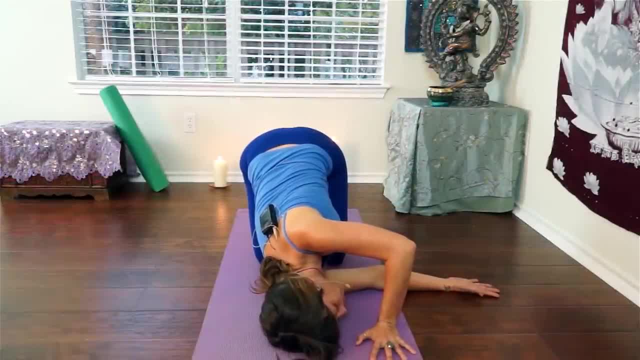 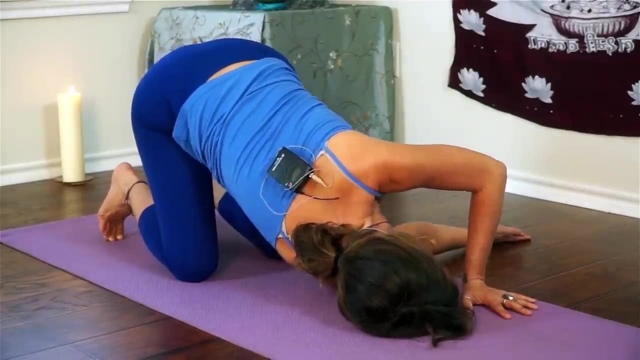 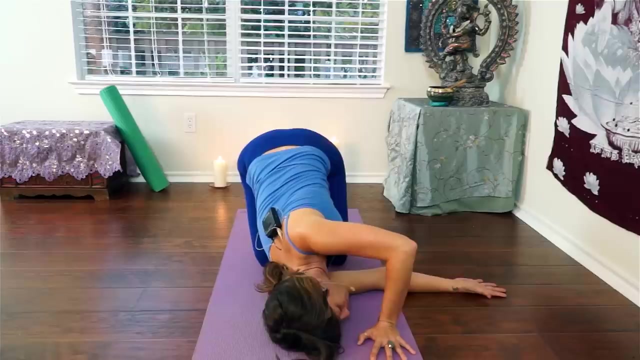 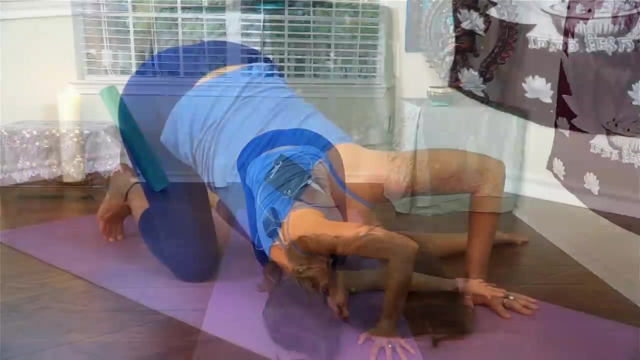 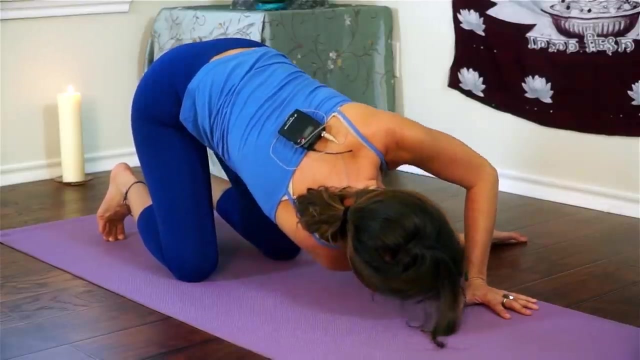 and you can bring your head down too. so now you have a twist in your spine and stretching into your upper back, reach across with your right fingers, really stretch and slowly press yourself back up- nice and easy- and bring your right arm up to the floor and bring your right arm up to the floor. 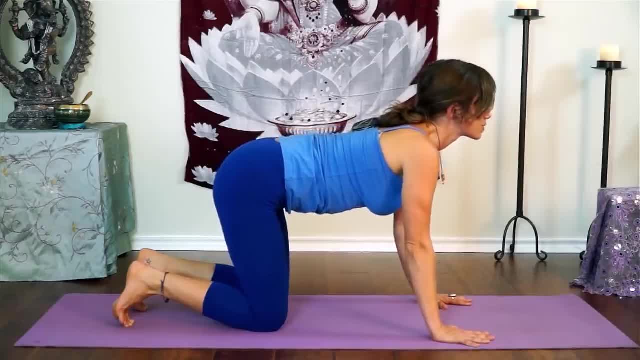 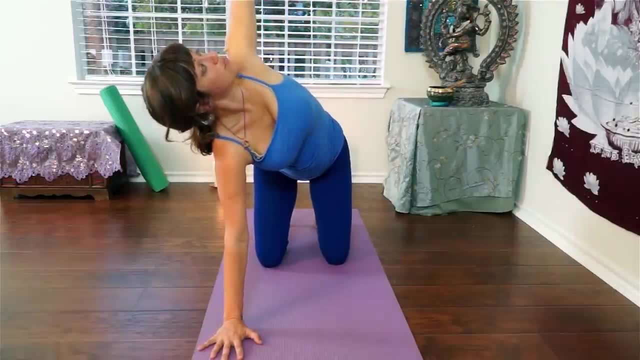 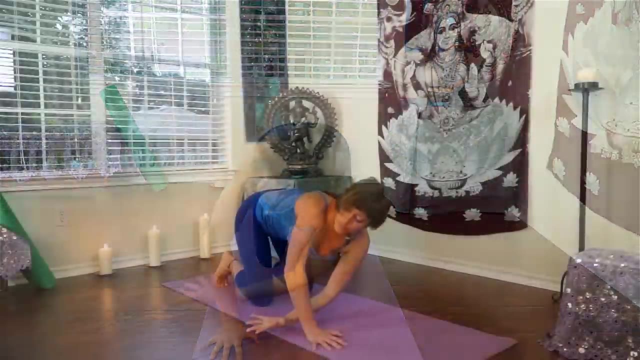 and bring your right arm up to the floor and bring your right hand back down to the floor and we'll switch sides. sweep your left arm up open through your chest and then sweep your left arm underneath your right arm, bring your shoulder to the floor and bring your head all the way down. 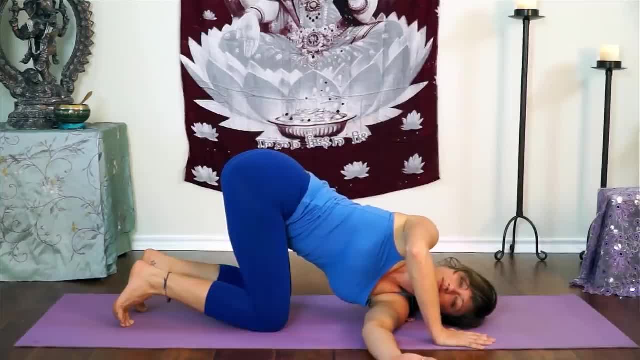 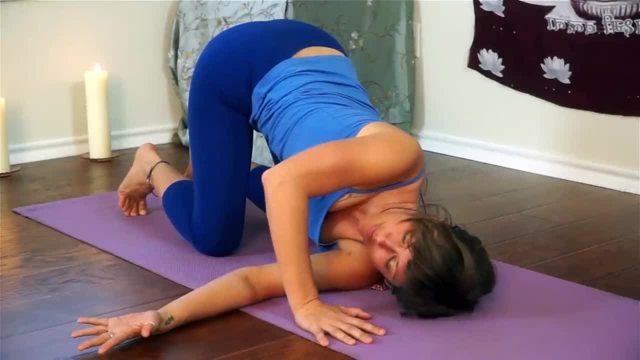 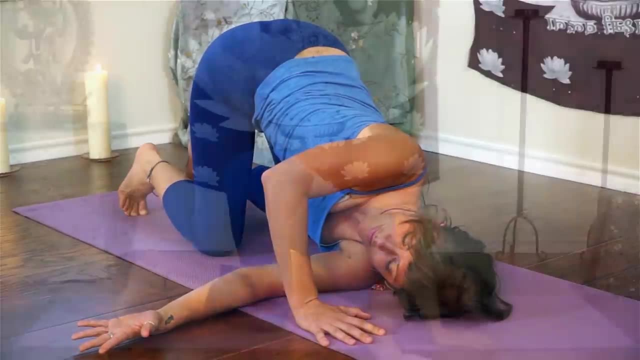 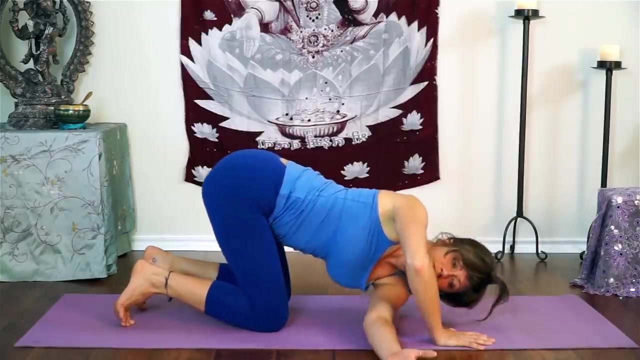 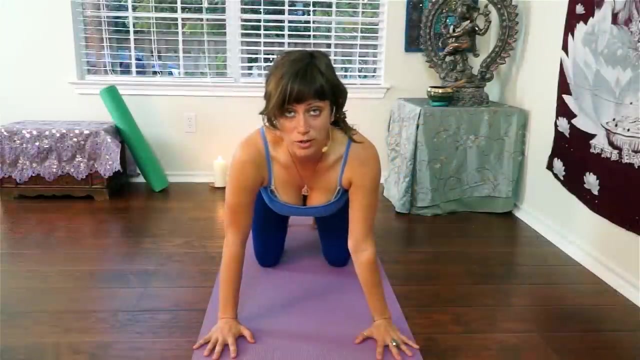 the right arm and shoulder down to the floor and we can slowly cut our wrist and slowly come all the way back. bring both hands down, bring your shoulder to the floor, bring your right arm up. we'll take a small child's pose here. so sit your hips back towards your heels. 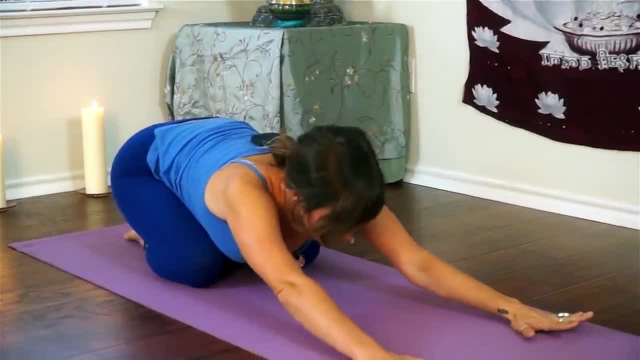 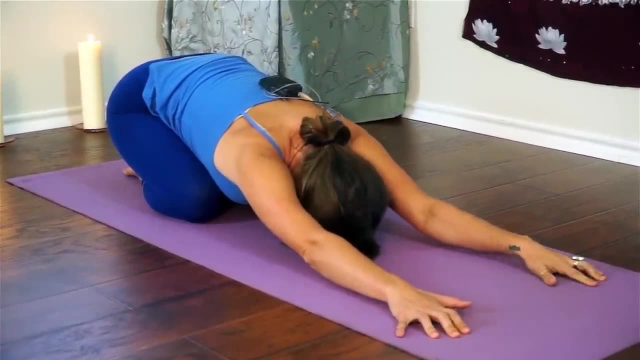 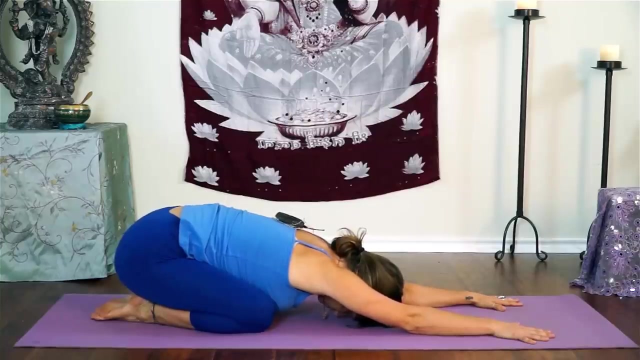 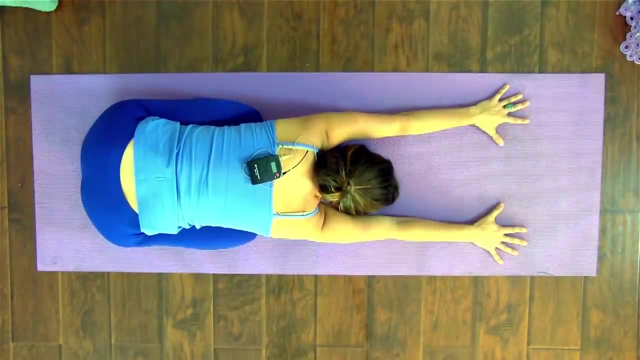 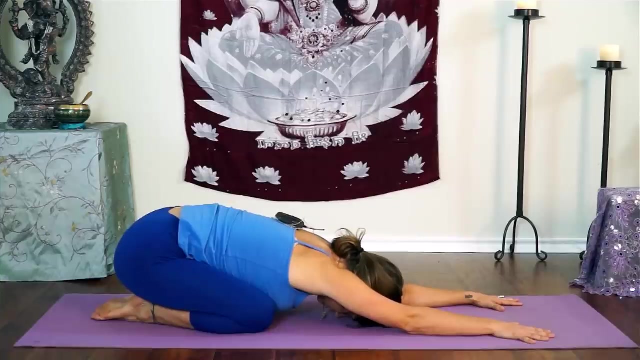 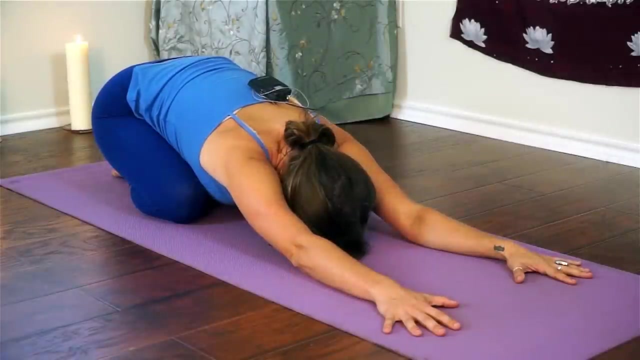 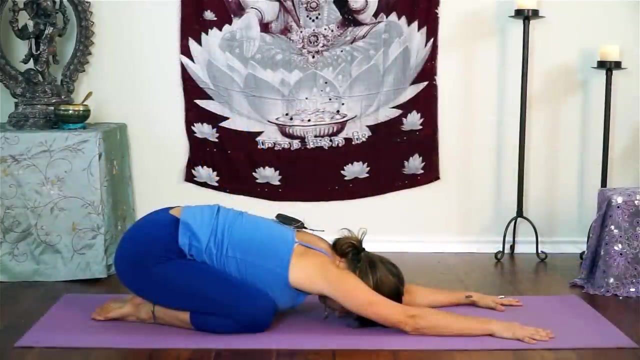 bring your forehead towards the floor. reach your hands forward as far as you can, so you'll have a gentle stretch through your shoulders as much as you can. let your hips sink down towards your heels. feel the length that's created along your spine. keep breathing deeply as you settle for a moment in this restorative pose. 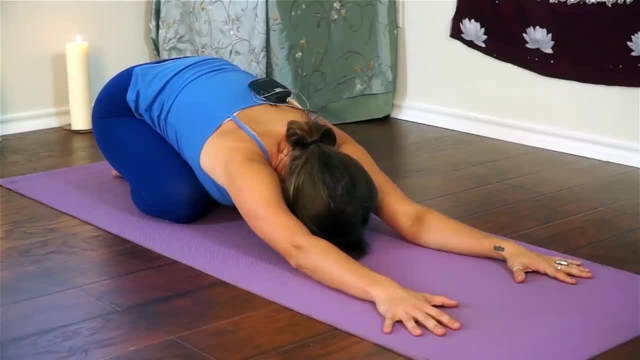 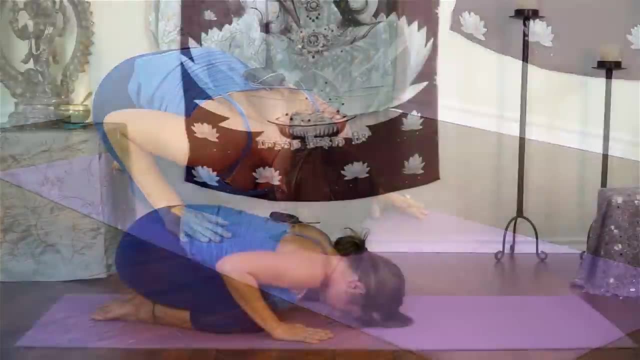 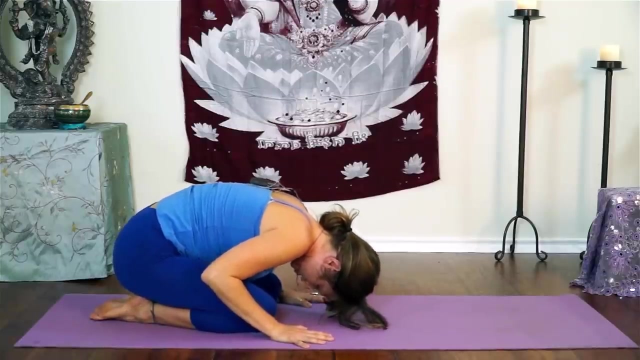 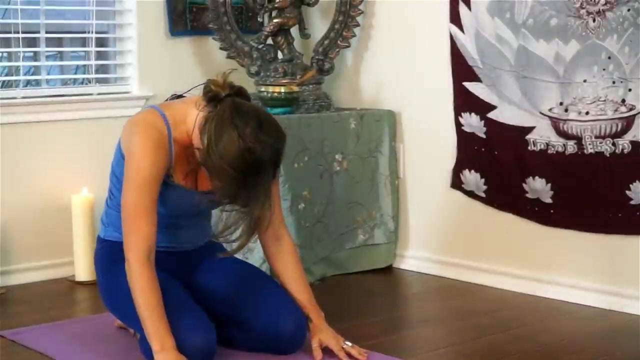 at the end of your exhale, start to press yourself all the way up, draw your hands in and roll up your spine, just like we did before. slowly start by stacking your vertebra, one at a time, one on top of the other. your head will be the last thing that. 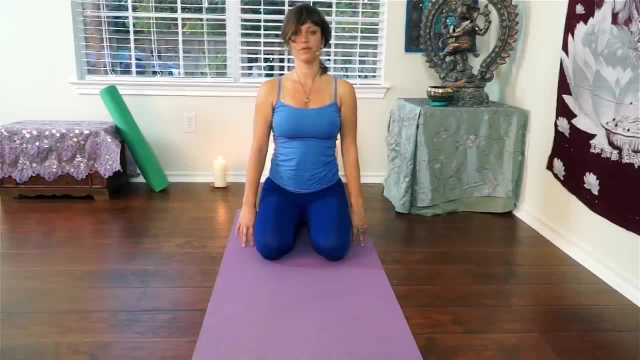 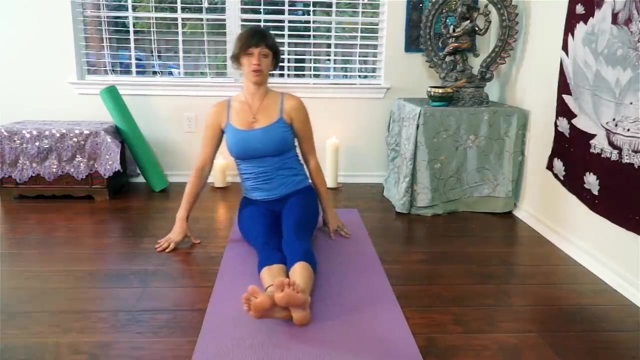 comes all the way up and you'll find yourself again in that nice, strong, centered posture. now we're going to make our way onto our back, so sit your hips over to one side so you can bring your legs around in front of you, and if you're on a yoga mat, like me, 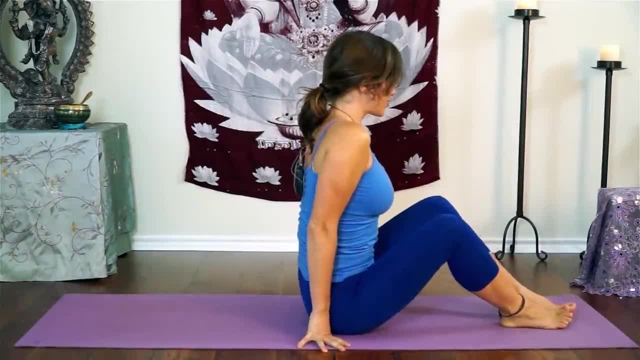 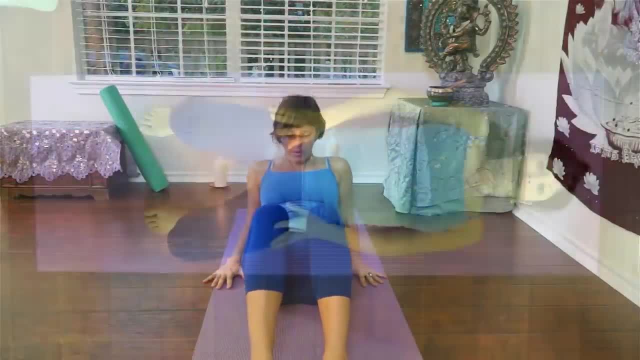 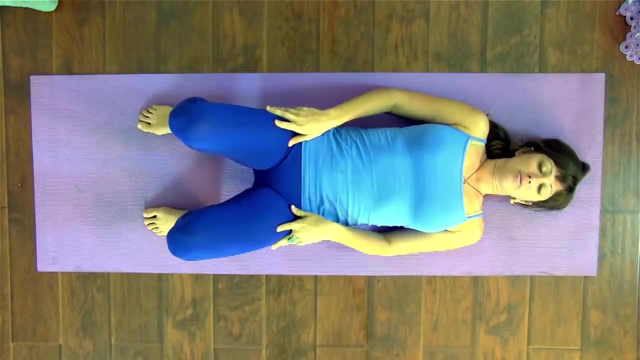 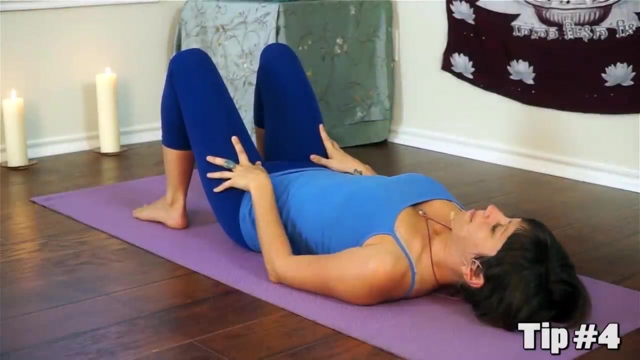 you might scoop forward a little bit, but if you're just in your living room or somewhere, you can just lie down right where you are. so once you are on your back, bring your feet flat on the floor and your knees up to the ceiling, and I'll mention. my next tip for reducing your back pain is to do: 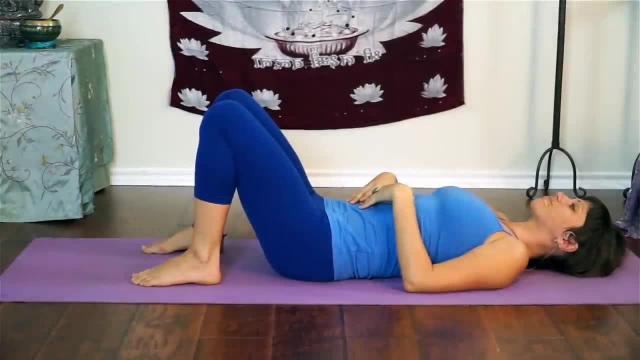 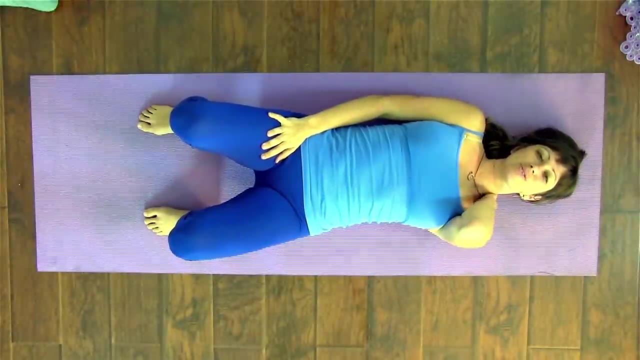 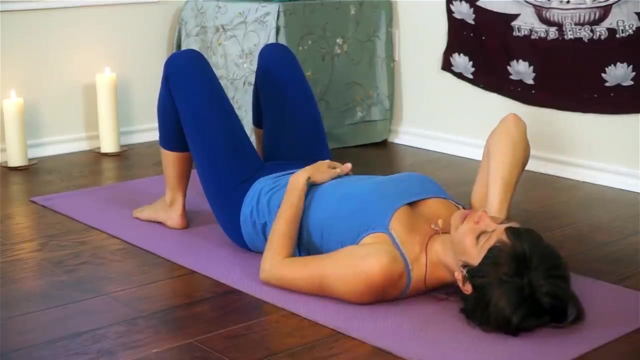 some self massage so you can use your hands to massage your traps, the tops of your shoulders, if that's an area where you get a lot of tension, so you can just squeeze those muscles and it can really help to increase the blood flow. you can also squeeze the muscles in your neck if you have a lot of headache tension. 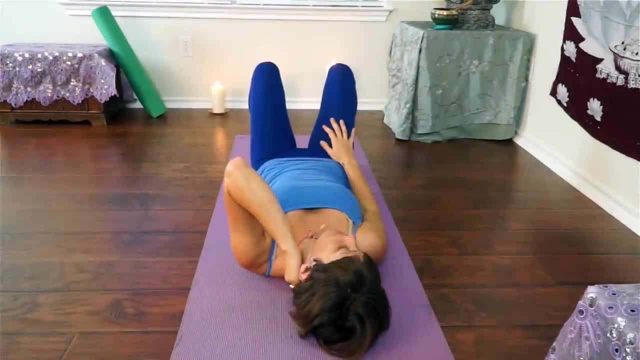 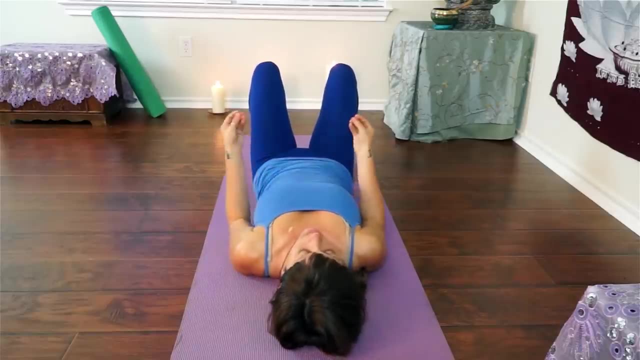 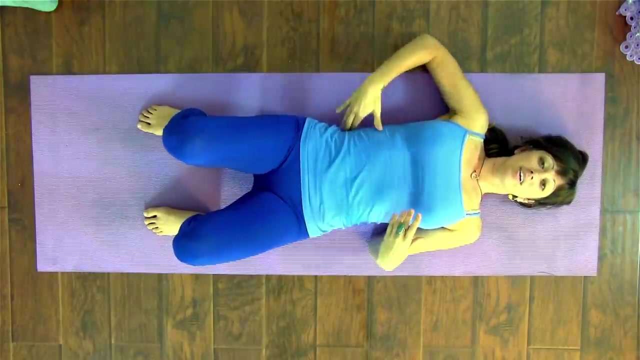 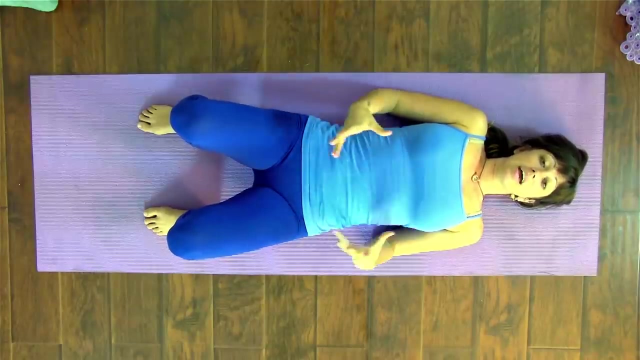 you can also squeeze the muscles in your neck. if you have a lot of headache tension, this could be helpful. another great self massage technique is to lay on a tennis ball or a pair of rolled up socks, so you can put the tennis ball underneath your spine anywhere that you have tightness or tension and laying on. 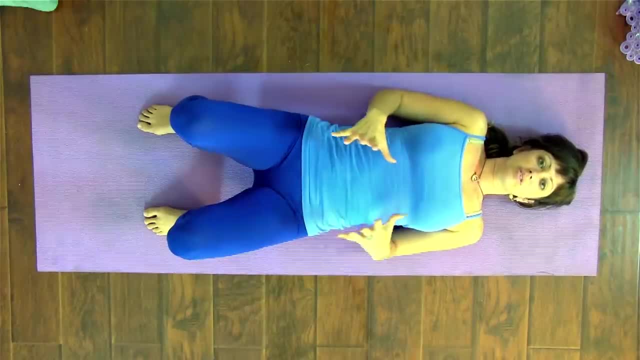 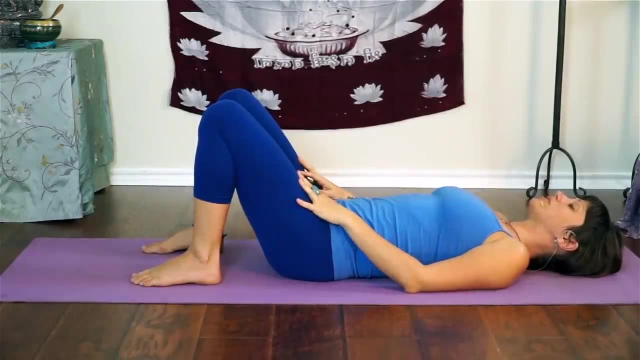 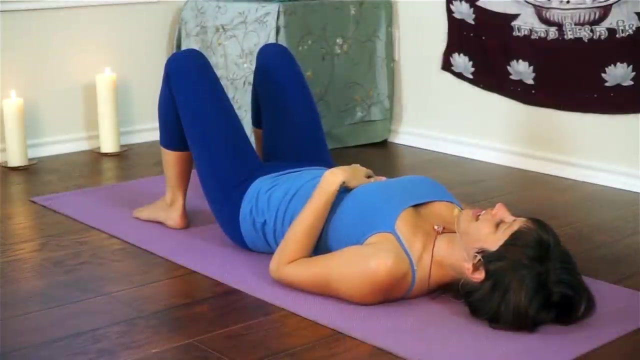 that tennis ball will also help to put some nice pressure in there and help relieve some tension. foam rolling is another great way of self massage that helps to relieve tension and ease back pain. so finding ways to massage yourself is an awesome way to reduce back pain. and our next stretch here I'm going to 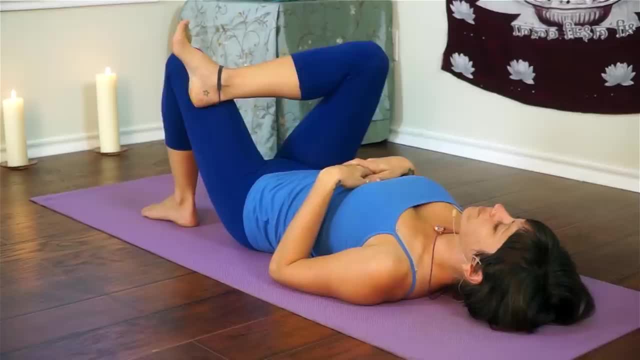 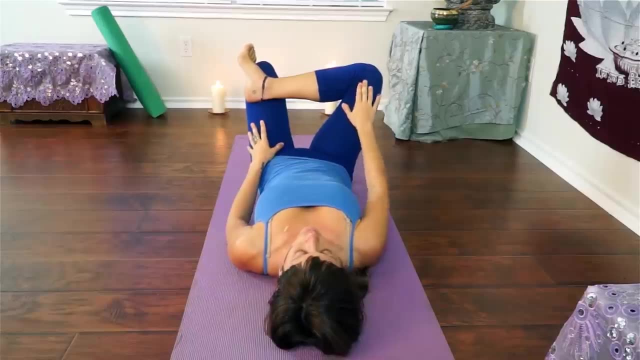 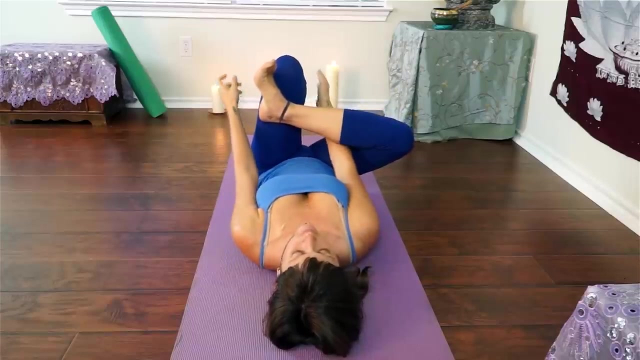 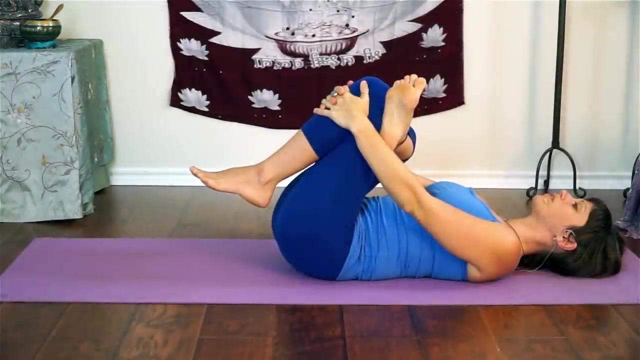 bring your right ankle over your left knee and press your right knee out towards the side. once you have this shape in your legs, draw your left knee in towards your chest and you can reach to grab around your knee. so this is going to stretch into your hips a little bit. so maybe you're. 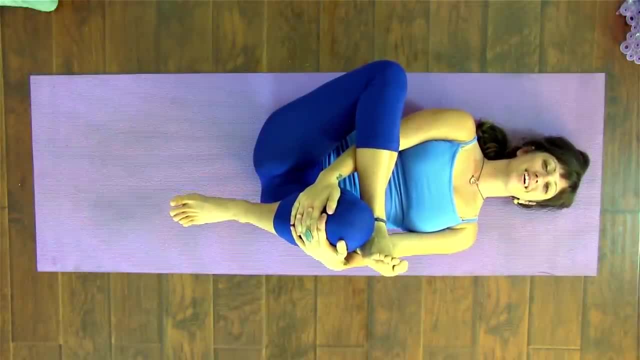 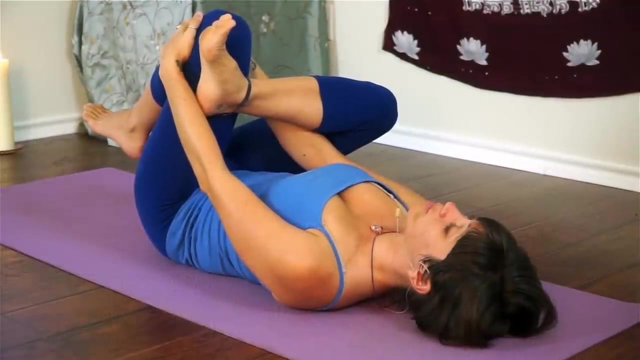 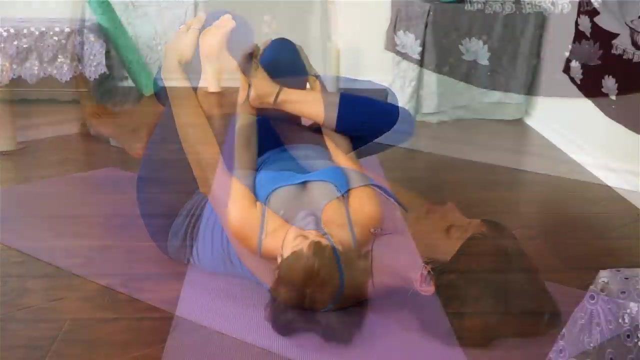 wondering: why are we stretching our hips? I thought this was for back pain, but the truth is that your glute muscles are one of the largest muscle groups in your body, so when those muscles get tight, they have a direct effect on what's happening in your spine. so, keeping your hips stretched out and 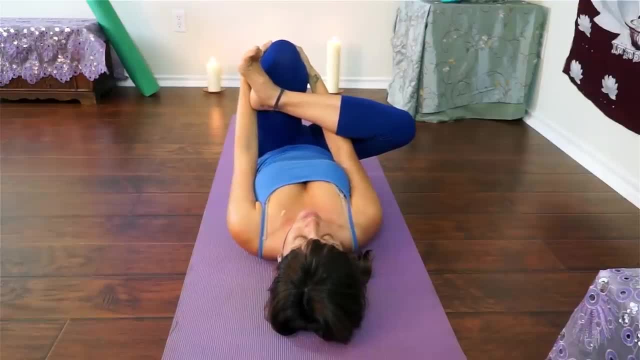 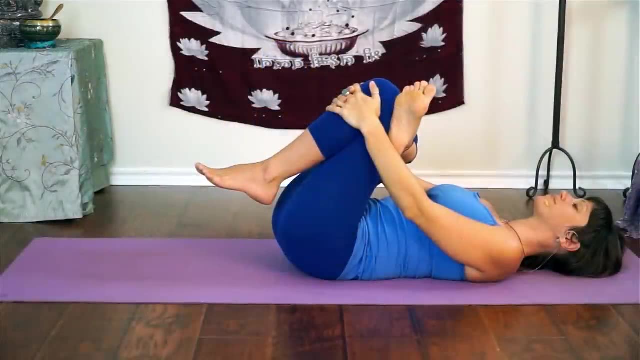 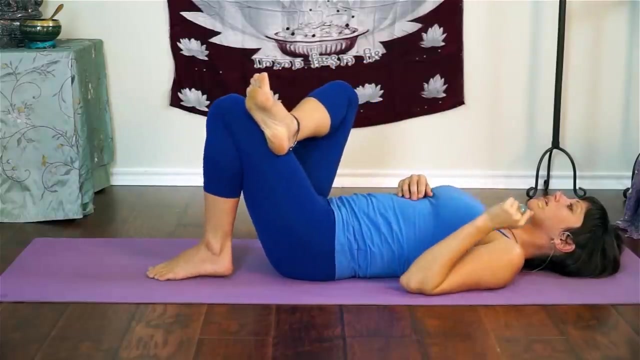 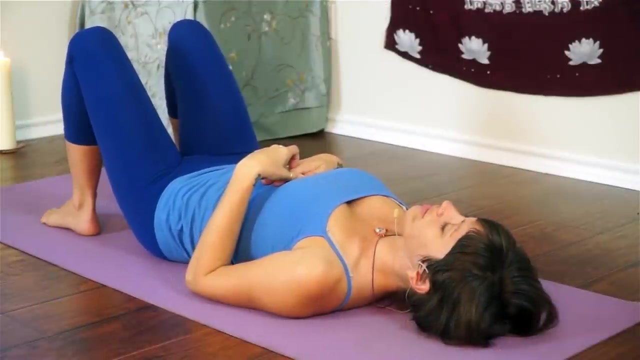 opened up, it's really going to have a powerful effect on cutting into the neck properly, impact on the health and alignment of your spine. so we'll switch to the other side. just release your left leg down and bring your right leg down and just notice the difference here and then cross your left ankle over your right. 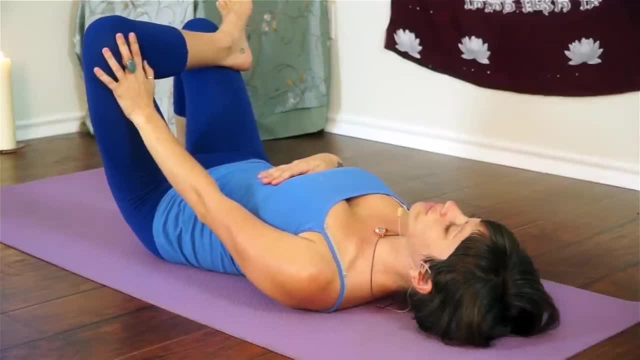 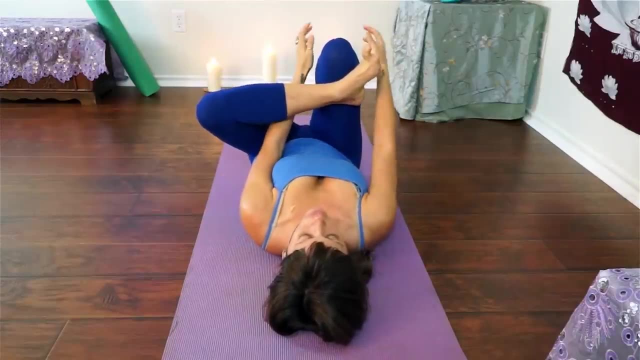 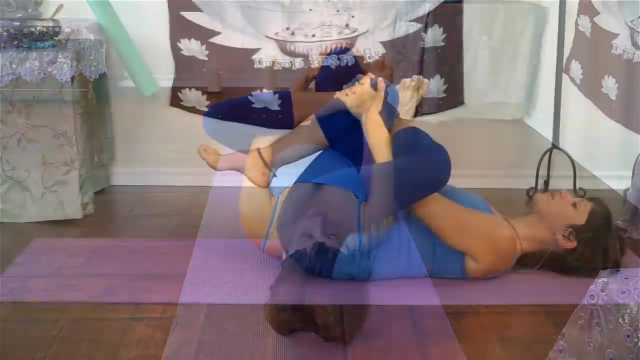 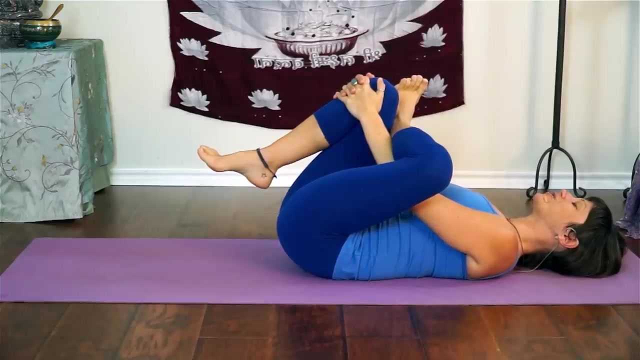 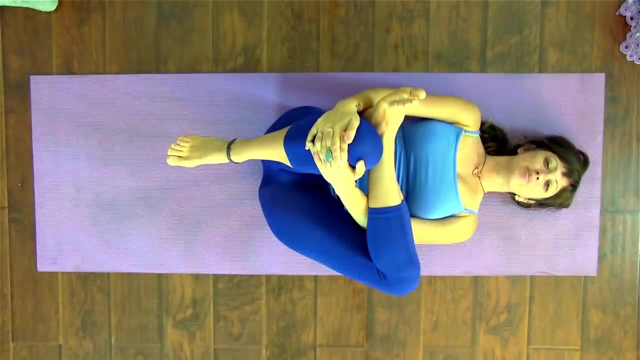 knee, press your left knee out towards the side and draw your right knee up towards your chest. try to reach for your knee, to grab and pull your right knee closer towards your chest and I'll remind you again about taking those deep, conscious breaths. and it's our first tip of the day and most important one. we should remember all the 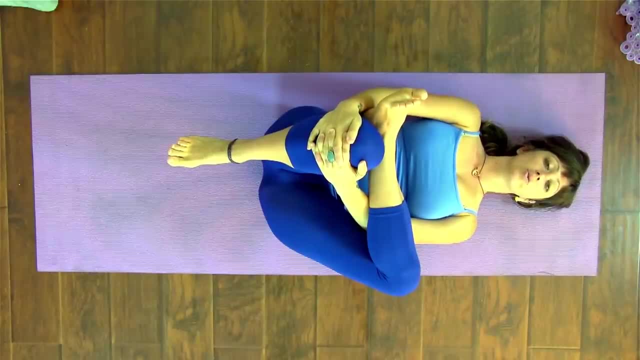 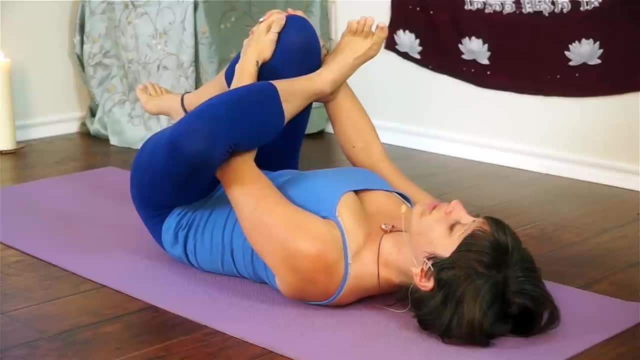 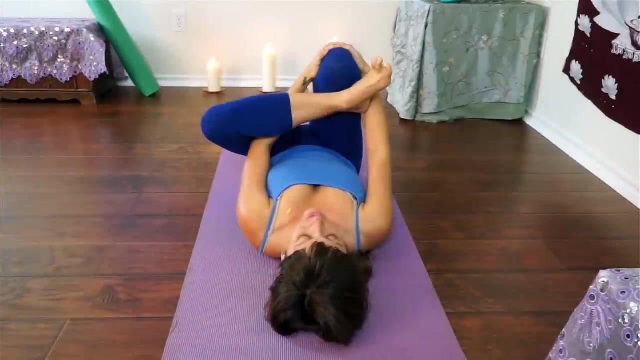 time. taking slow, full, deep breaths will help you to alleviate tension in your body and help to reduce your mental and emotional stress. so I can't say enough about the power of conscious breathing. so just take that big, full breath in, expand your belly. feel how good it feels. 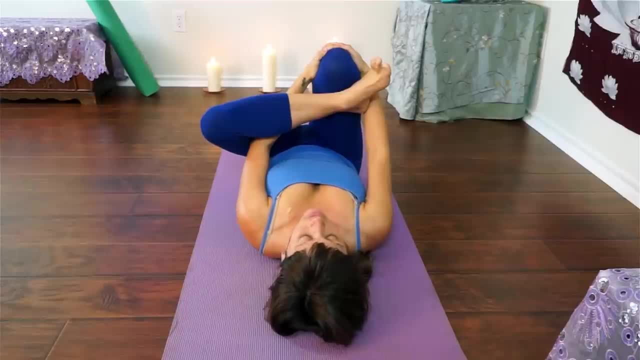 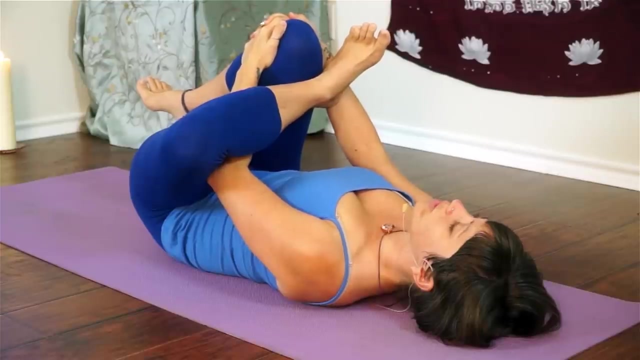 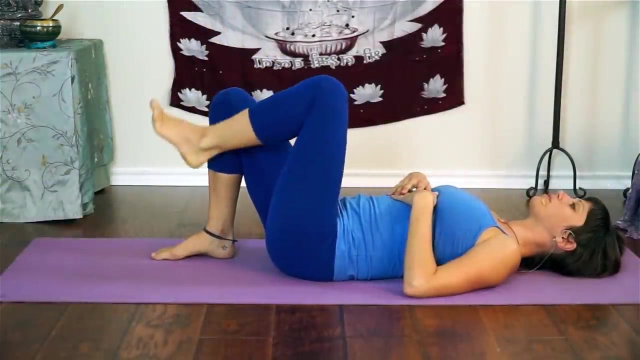 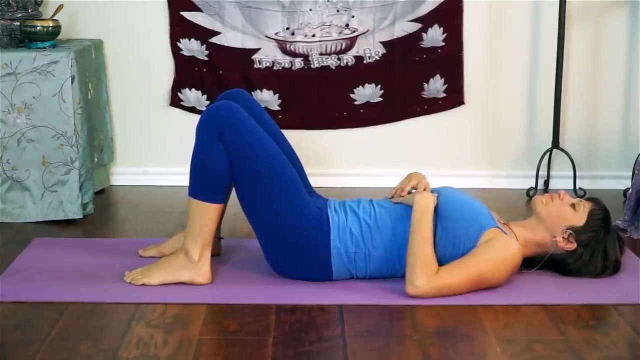 to breathe and exhale. just release any tension, any blockages. just let it go and let's slowly bring your right foot all the way back down and bring your left foot down. just feel your hips more open. we'll take one more twist here before we finish today. so extend your left leg all the way down to 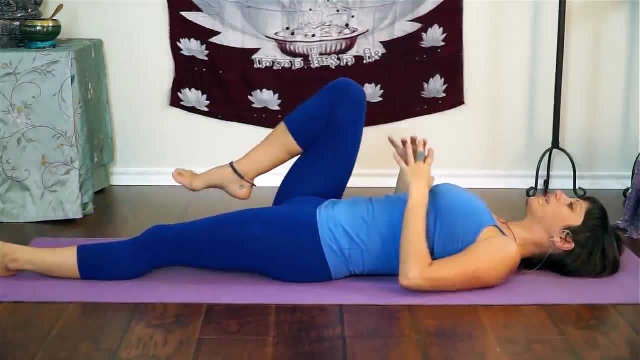 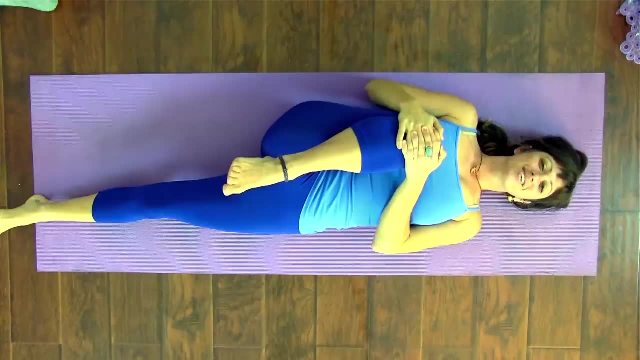 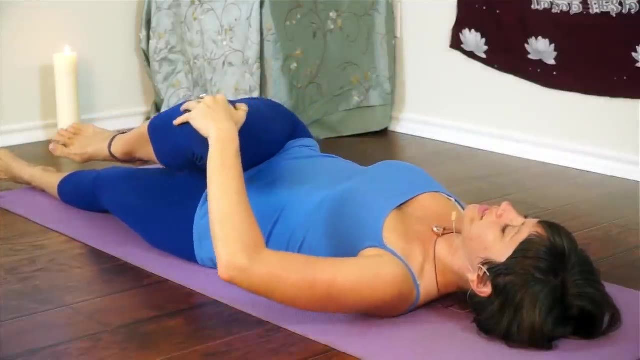 the floor, bring your right knee back up towards your chest and give it a little squeeze and twist your right knee across to the left side of your body so you twist all the way over. I got a little pop in my back. I think that's a good. 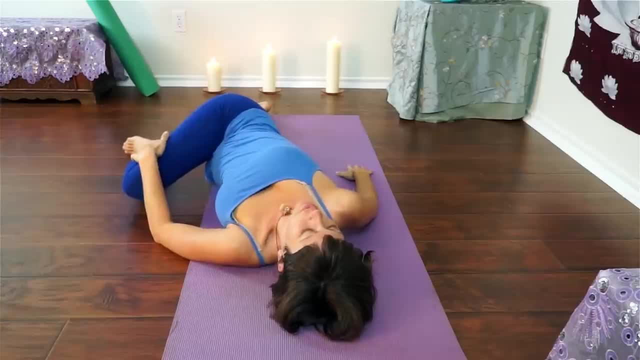 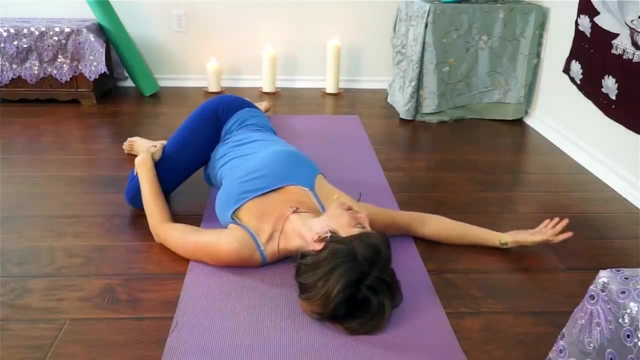 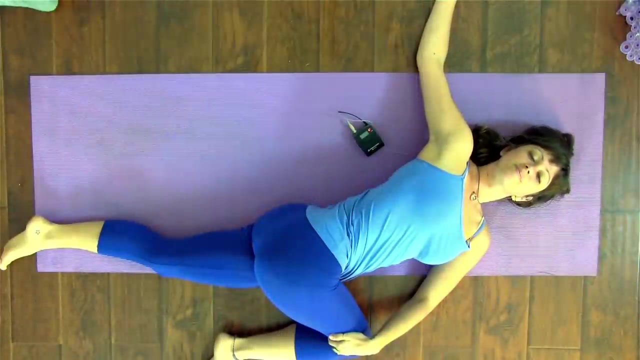 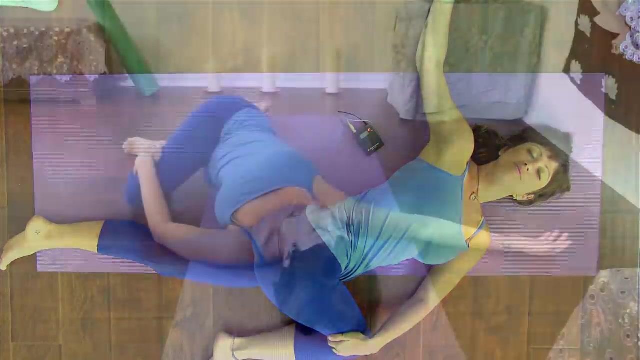 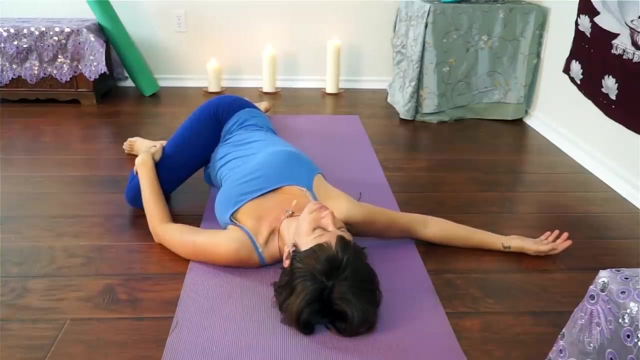 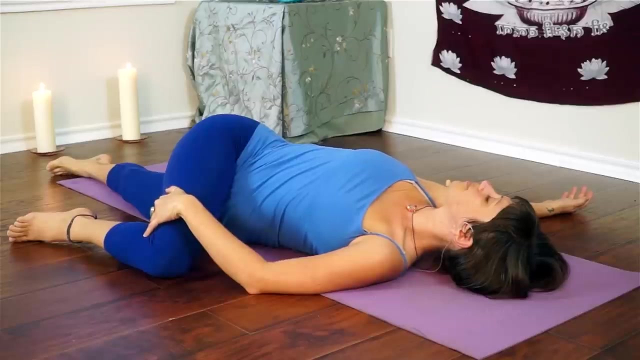 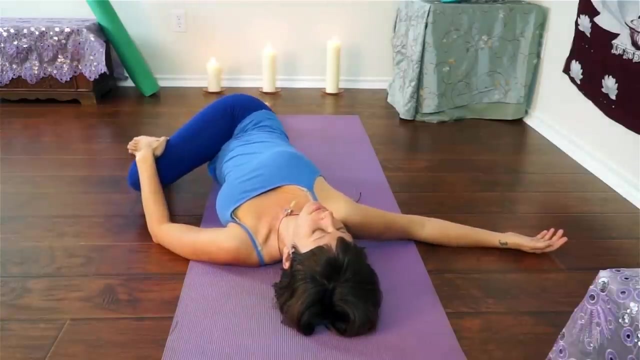 sign. so you twist as far as you can, then open your right arm out to the right side and you'll get a little twist and you'll get a gentle stretch across your chest. let's slowly unwind coming back to center, roll all the way back onto your. 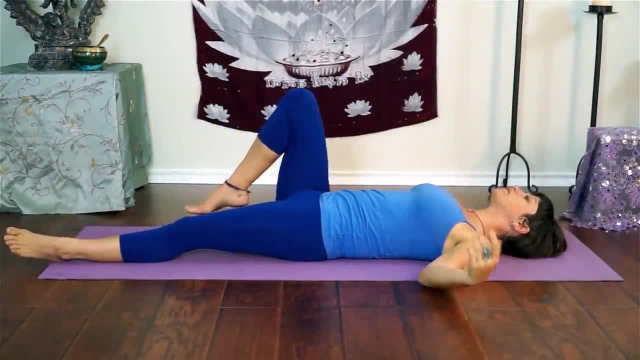 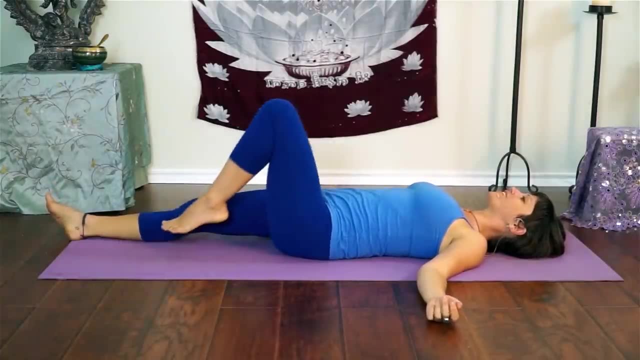 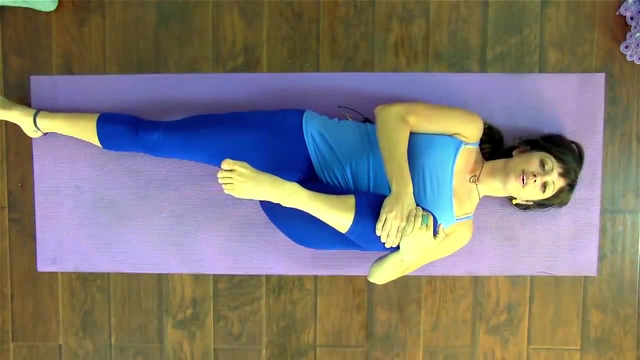 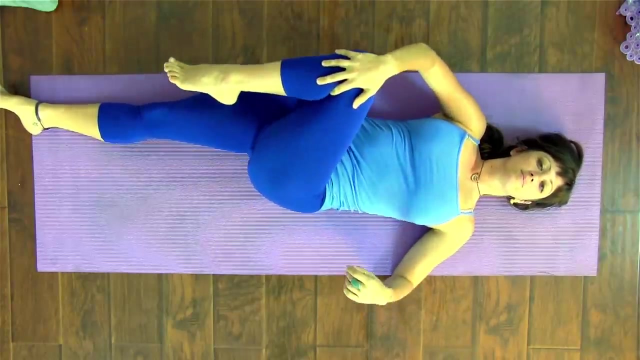 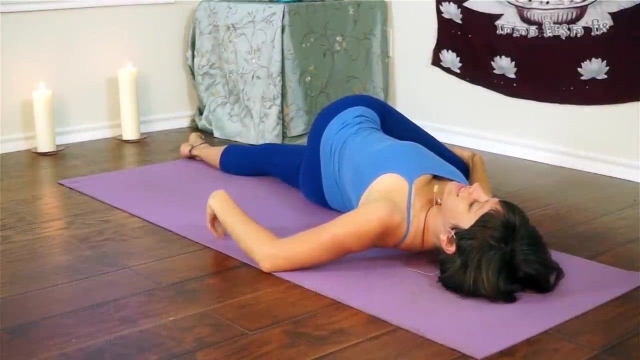 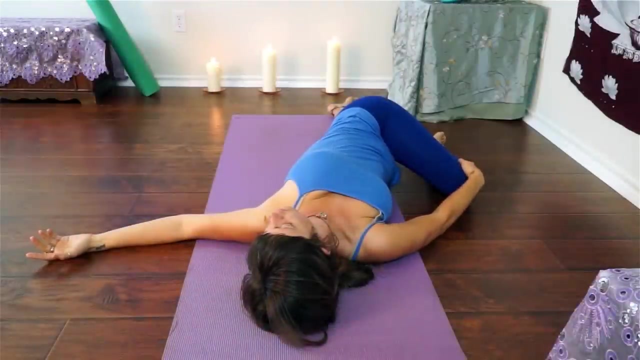 back and extend your right leg all the way down. then bring your left knee up towards your chest, squeeze it in and twist your left knee across to the right side of your body as far as you can, and extend your left arm out to the side for a gentle stretch in your chest. 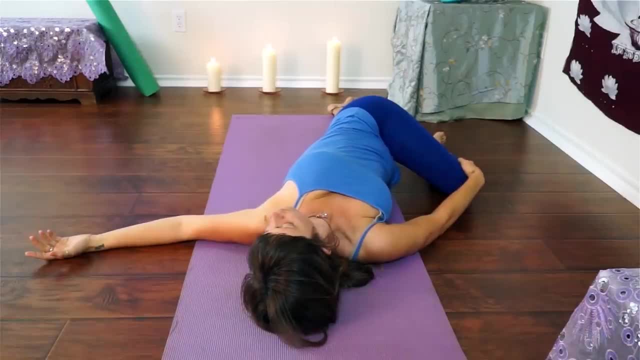 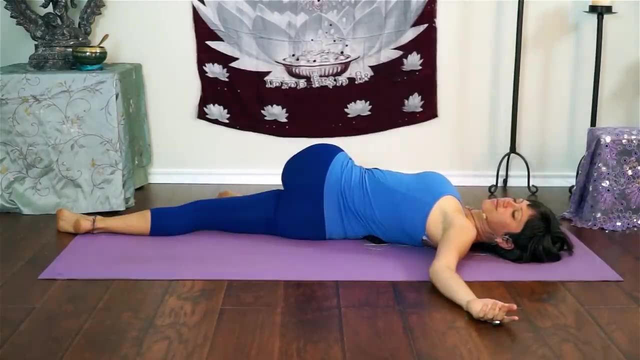 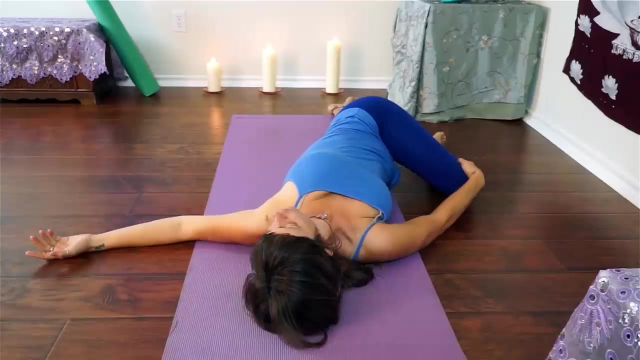 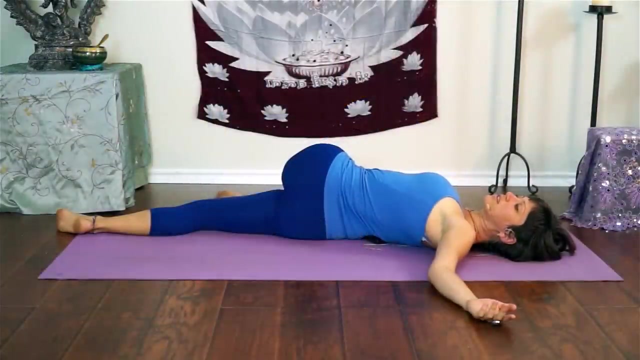 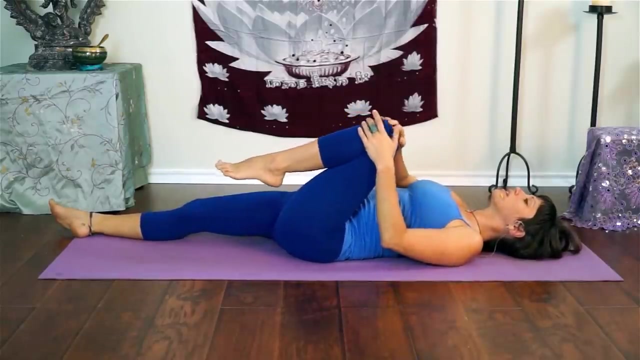 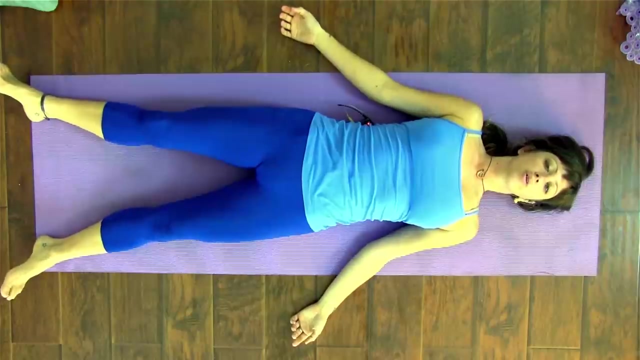 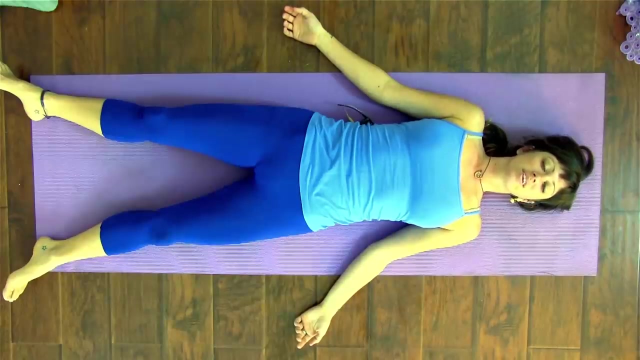 and, and and. Thank you. And let's slowly come back to center, rolling onto your back and extend your left leg all the way down. Let both arms come down by your sides, Let your palms rotate up towards the ceiling, Let your breathing be slow and deep. 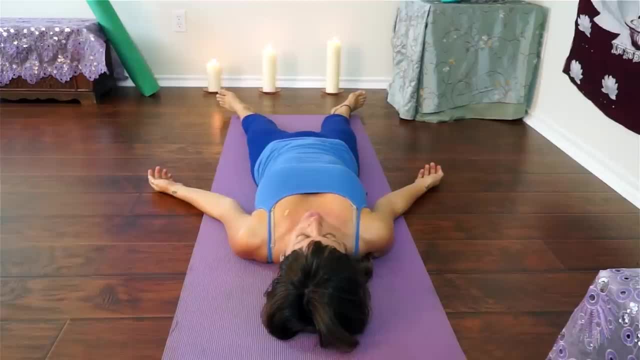 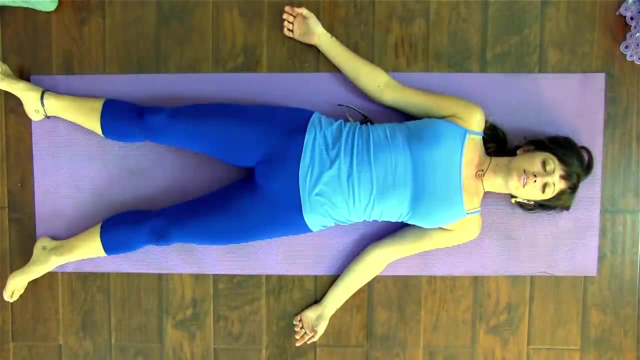 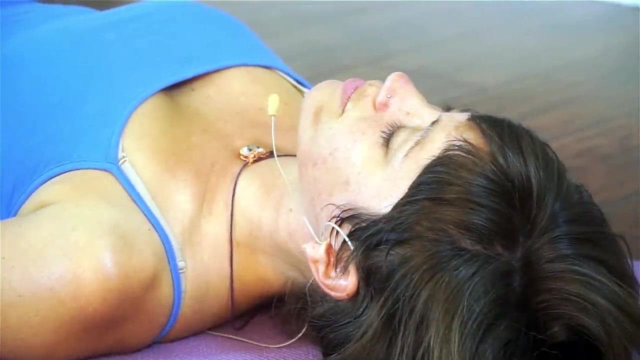 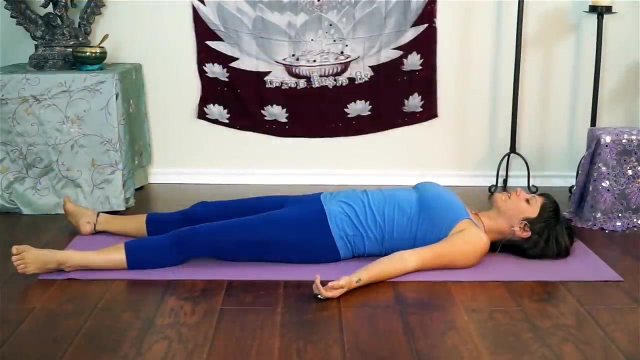 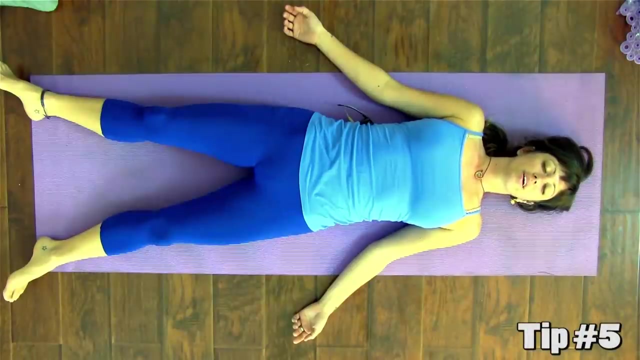 And gently close your eyes. Take a moment here to notice how your back feels differently than when we first started. Let yourself rest And we'll finish with our final tip for relieving your back pain. It's just simply to favorite this video and come back and practice a few times a week. 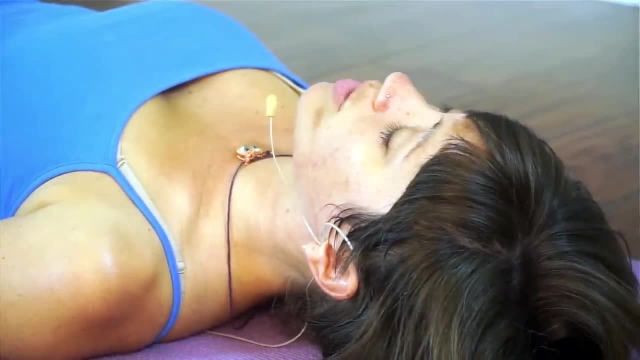 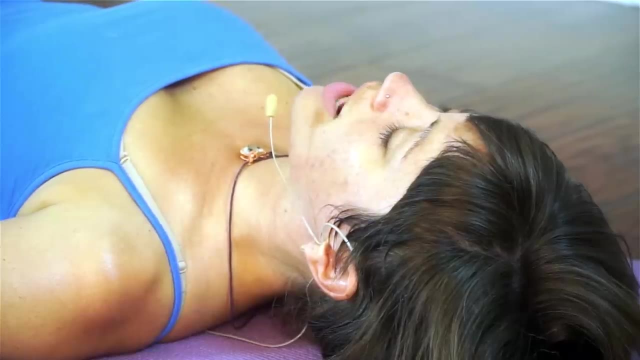 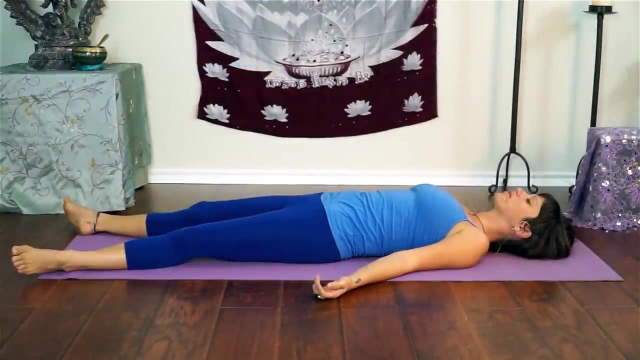 I'm sure by now you can feel the benefit of this work. So the more often you can practice, the more it's going to reduce your pain, And if you can remember some of these easy stretches, you can do them anytime, anywhere. 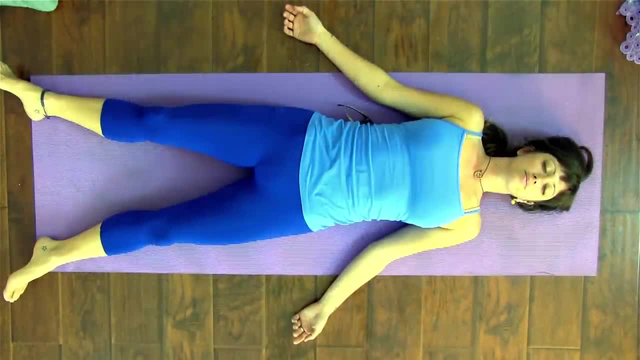 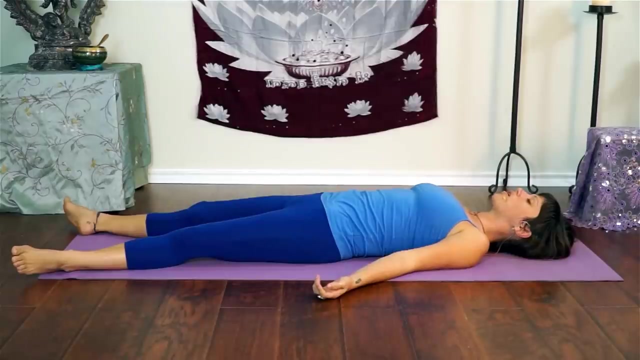 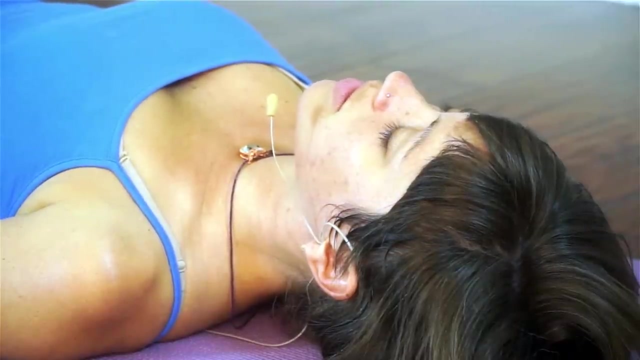 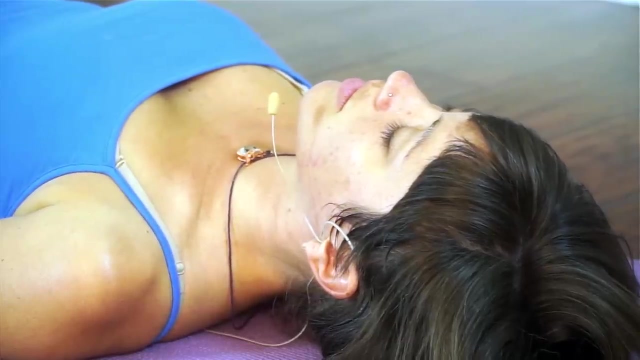 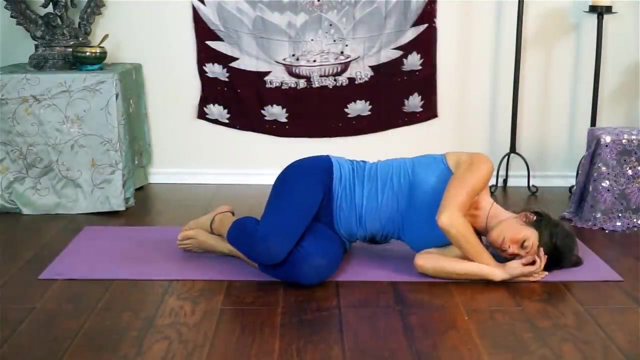 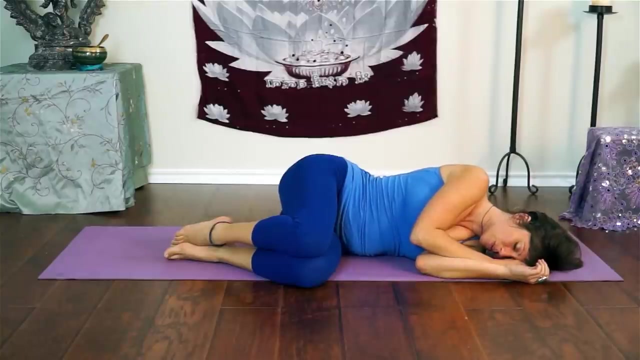 Thank you for watching. Thank you, Feel free to stay and rest as long as your body needs And whenever you're ready to come back up, start by rolling over onto one side, coming into a comfortable fetal position. you can take a moment to rest here, feeling nurtured in this space, and to come up use. 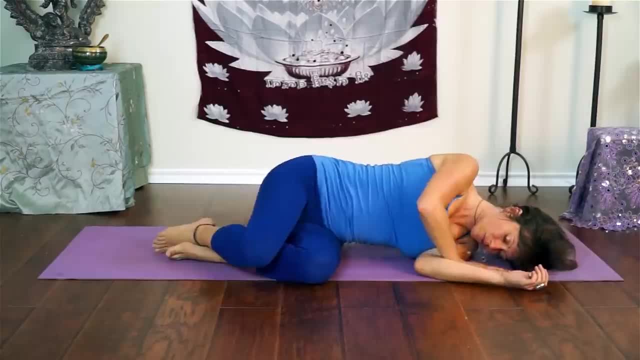 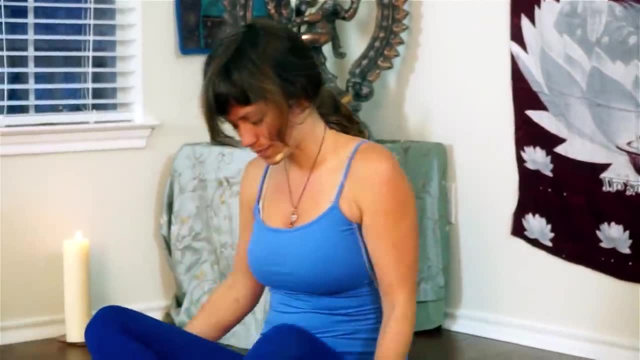 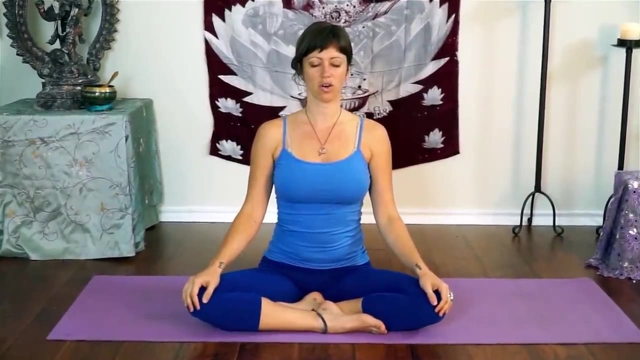 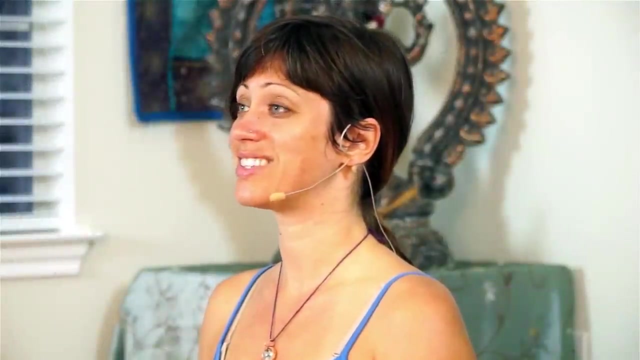 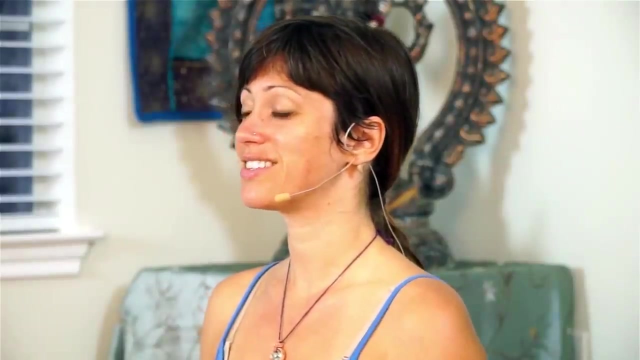 your top hand to press down and push yourself up to a comfortable seat. so, as you sit all the way up, return to this nice tall, supported posture that we've been practicing today and notice how it's easier now than when we first began. bring your hands to a prayer. 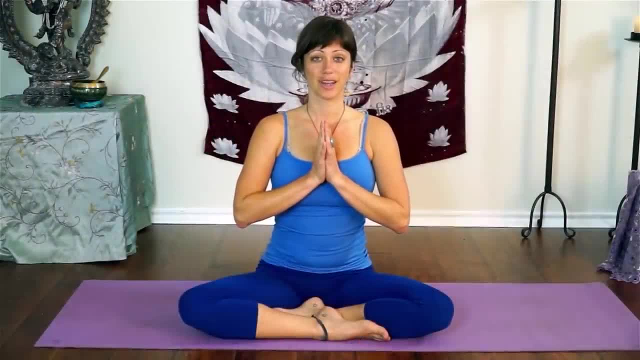 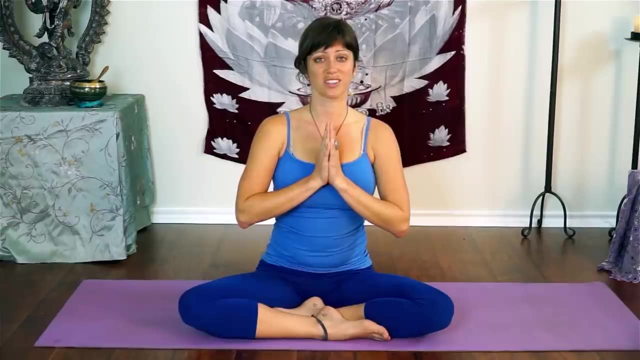 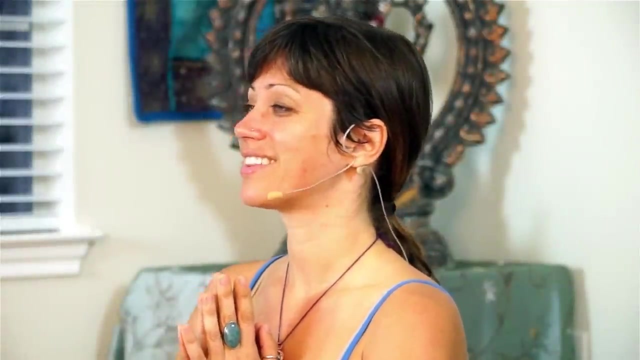 position at your heart and bow to the wisdom and light within your own self. give yourself some gratitude for taking this time to stretch and take care of your body and, if you haven't, leave me your comments below. I'd love to hear how this practice is helping.